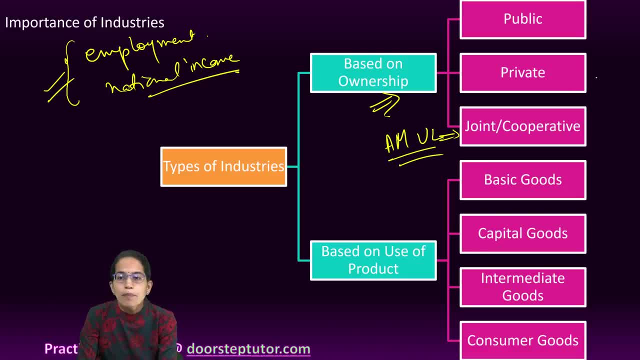 people come together and work as a unit. Public industry is an industry which is controlled and funded by the government. However, private is under a private control, So the industries which are meant for strategic purpose- defense, security- are mostly in the public sector. 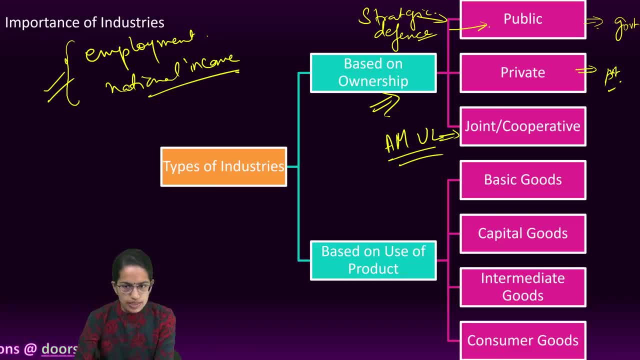 not just in India, but across the globe. That's a common phenomena that we witness. The next is the classification Based on the use of product. Now, it's very important to understand. this is how we write our answers. Let's say, you have a question on understanding the types of industries. We don't 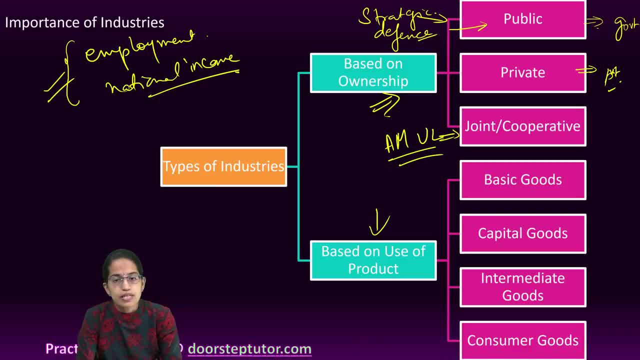 just put that. okay, there is a large-scale industry, small-scale, medium-scale private joint, but we rather classify it and subclassify it. That makes the content much more systematic. So here, based on the use of product, the industry can be called as a basic good industry. 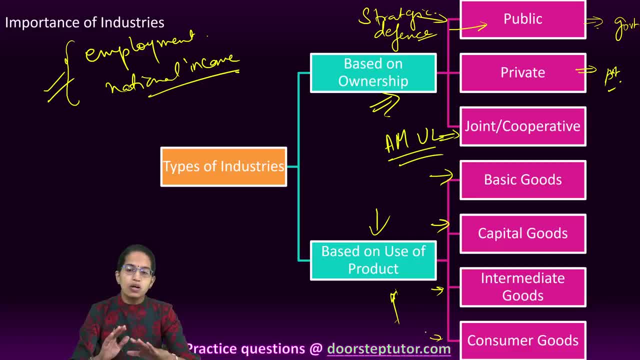 capital, good industry, intermediate and consumer goods. Now, what are the differences? Basic, good industry is an industry that manufactures the basic material. I want to establish an industry. Now, for that industry, I would require machinery manufacturing plants. What are those? Those are basic goods, which are: 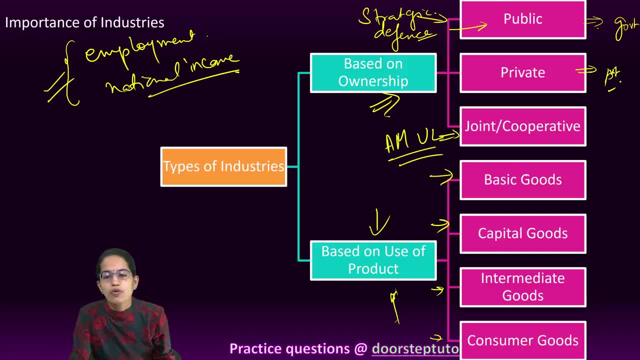 required for the functioning of the industry and therefore they are called as the basic goods. The next is capital goods. Capital goods are the assets, the building, the machinery, the tools, the vehicles. All these are capital goods, So they are there for a prolonged period. 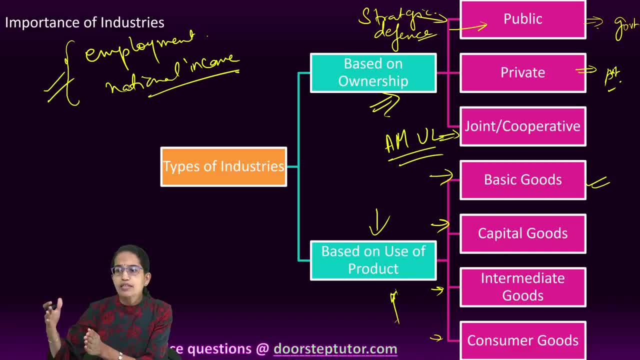 of time and they do not make the finished good. They are actually used in the process of making the finished good. Then the intermediate goods which are produced in the process of processing and finally the consumer goods which are used by the consumers, For example clothing, food. So 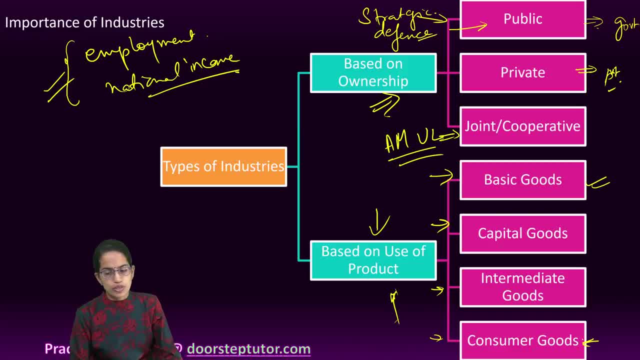 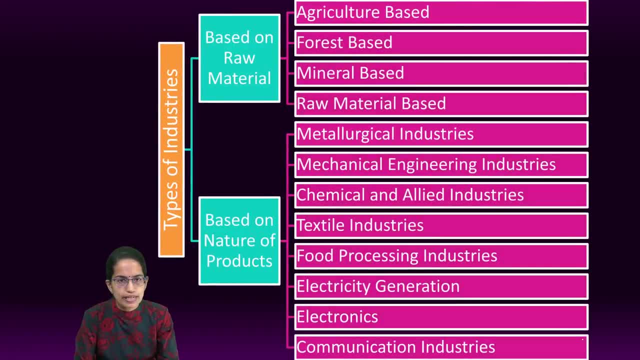 all those are consumer goods. Now the industries pursuing in those sectors are called as the consumer good industry. The next good classification is based on raw material. I can say an industry which relies on agriculture based products would be called as agro-based industry or 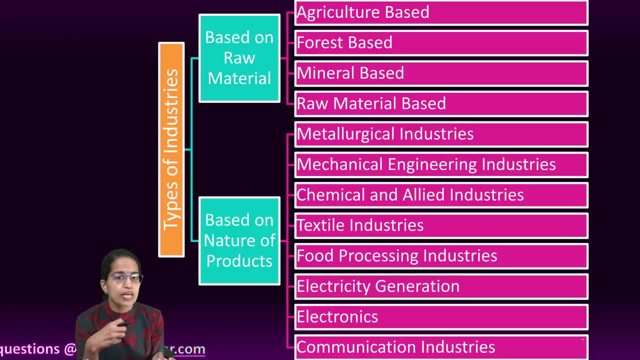 agriculture based industry. Cotton textile is a good example. We have mineral based industry, where we have iron and steel as a good example, Raw material based industry, which is based on raw material. Now raw material could again be from agriculture, from mining. So it's the 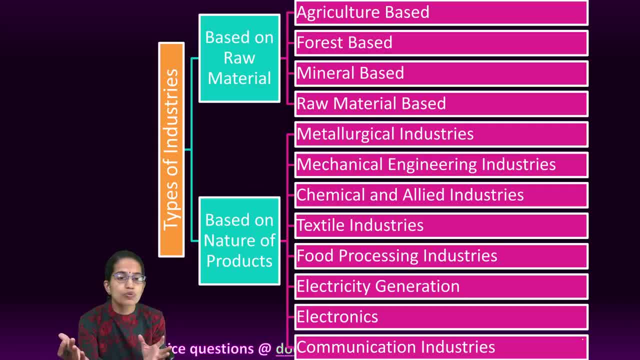 location that we would understand later is closer to the raw material. Then we do have forest based industry, where we have products from forest which are used in the process of industry. For example, manufacturing and selling of honey is a forest based industry. Now it could be small scale. 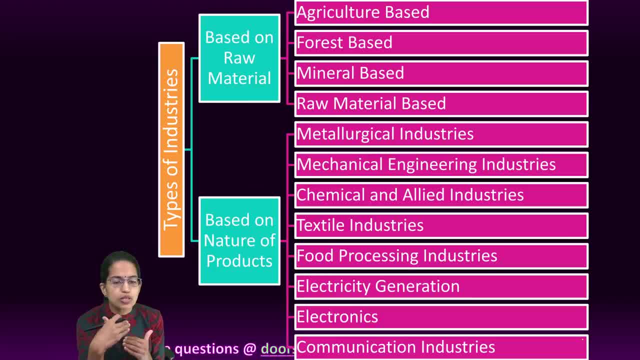 large scale or medium scale, based on the size. Based on the nature of products, we have eight further classification. It can be either metallurgical industries, which are used in the manufacturing of metals, mechanical engineering industries, chemical engineering, which are mainly allied to pharmaceuticals and the chemical compounds used for 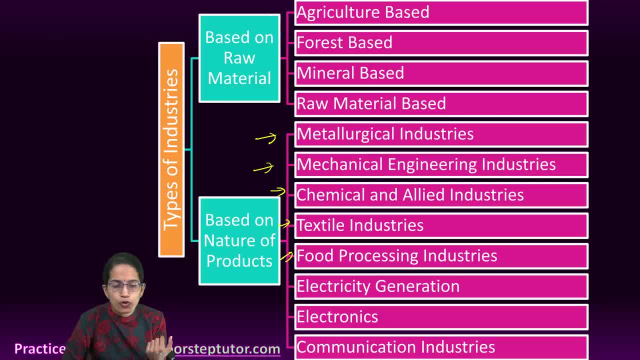 various purposes: textile, which is cotton textile. food processing, which is again the agro-based industry, electricity generation, electronics and communication industries. So that's another classification based on the nature of product. Now, coming on to the factors of location of an 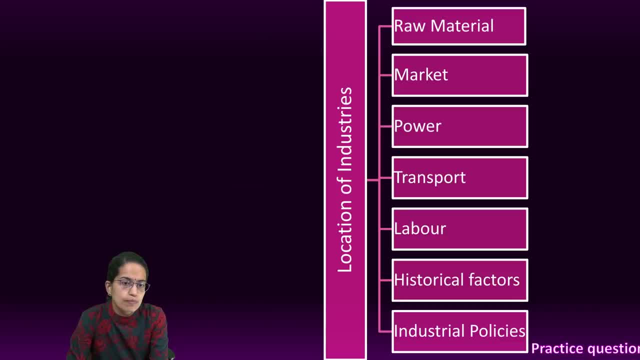 industry. Now again, this is a very, very interesting and an important topic to understand In the higher classes. as we go, we would understand a model which is known as Weber's theory for industrial location, One of the most common and popular theories under industrial location. But we do have 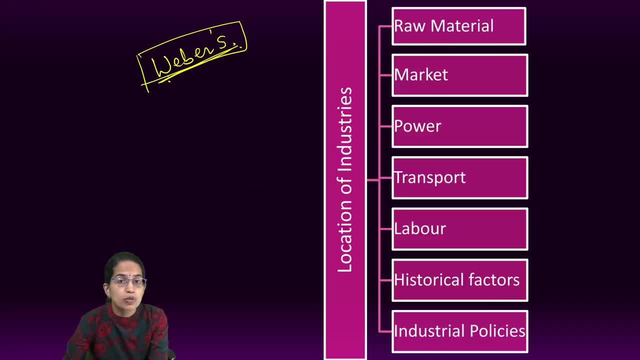 other scientists and other geographers as well, who have laid down the localization theory. But what is the localization theory? Well, the localization theory was the location triangle, and this triangle talked about where the industry would be if there are raw material and finished product. Now the 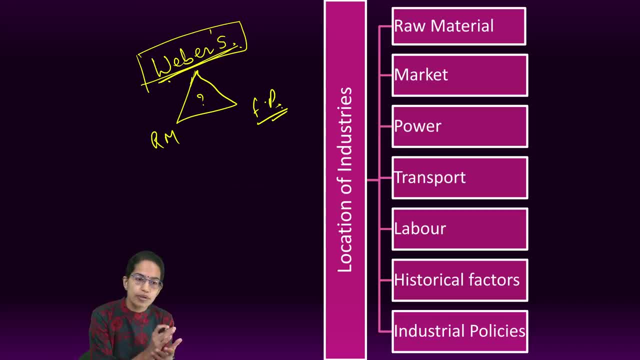 industry where raw material is heavy. In that case the industry would be close to the raw material. For example, iron and steel uses lots of iron, lots of coal, which is bulky to transport, and therefore the industry would be most probably near raw material. 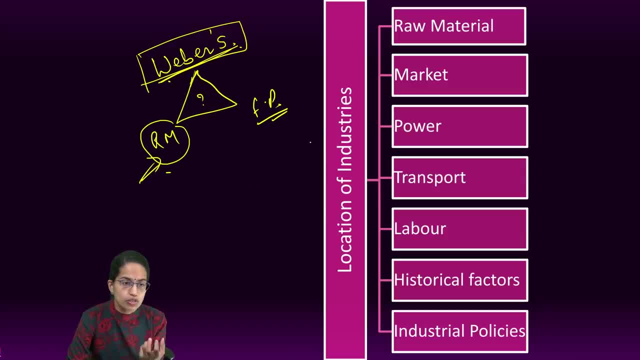 Now, if you have textile industry- Now cloth being manufactured from cotton. Now, once you have the cotton yarn with you, where could you have the cotton textile industry? Probably close to the market, So you would have better reach, better availability. Now industries which are weight, losing Weight. 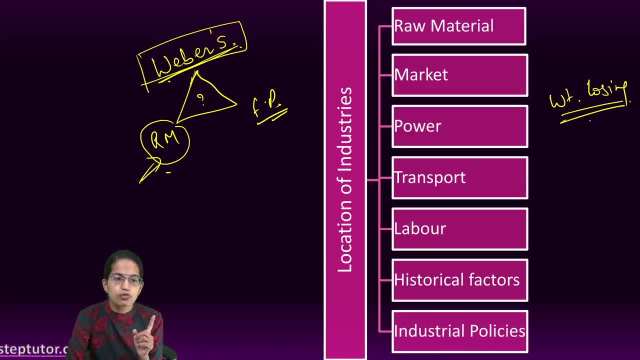 losing. that means they lose weight in the process of manufacturing, For example, iron, steel, sugar cane industry, paper and pulp industry. All those weight losing industries are located close to the source of raw material. So, as I said, iron and steel industry is a good. 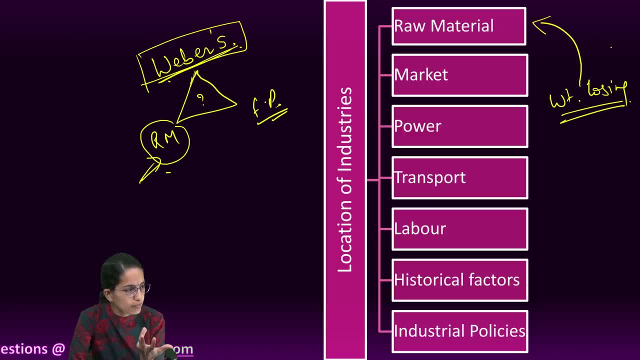 example, Paper and pulp industry, sugar cane industry, sugar being bulky to transport- All those are located close to the source of raw material. Now for iron and steel we would have a separate case study, But to understand that for optimum use they are located close to: 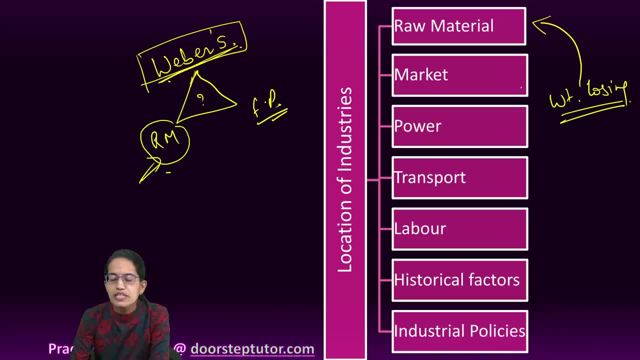 not only the iron fields but also the coal fields. Major coal fields in India are in Bokaro, Durga, Dharpur. Then we have iron ore from Badravati, Raul, Kela, Bilai. So the industries would be. 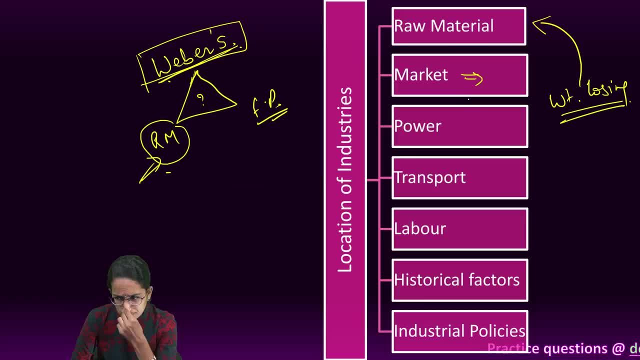 closer to those locations. Market, as we said, heavy machine tools, anything which is non-weight losing. So weight losing would be close to market. Non-weight losing would be close to market area, Clear. The next is power, For example, aluminum industry. we have synthetic nitrogen industry. 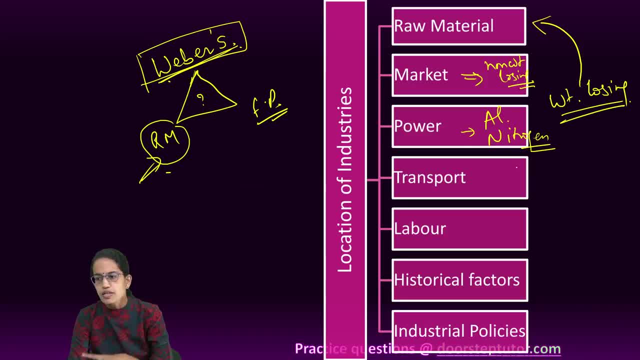 Both of those industries are closer to the source of power because they require huge amount of energy in them in the processing, And therefore aluminum and synthetic nitrogen are two typical industries located close to power. The next is transport industry Now location because of transport. 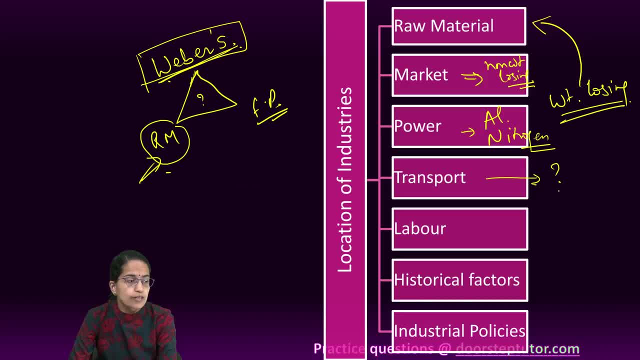 Now we do understand that transport is a bigger cost. So if the cost of transport is too much, then it would definitely have an impact on the final product. So we ensure that the cost is remained optimum so that the product price, which is finally there, 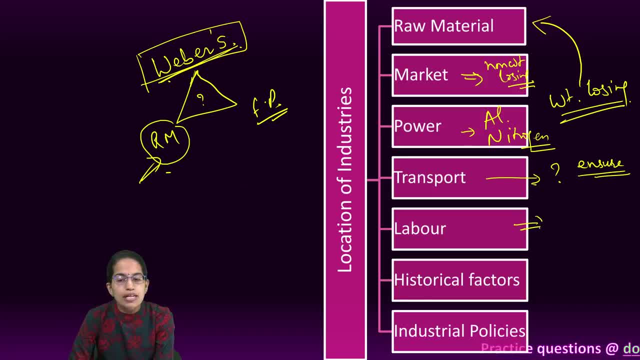 after processing is not extremely high. Similarly, labor- Cheap labor is one of the factors which decide the localization of industry. Government over the years gave numerous incentives to establish industries in the remote and the tribal pockets, And one good advantage of it was cheap labor which was available. The next is historical factors, For example. 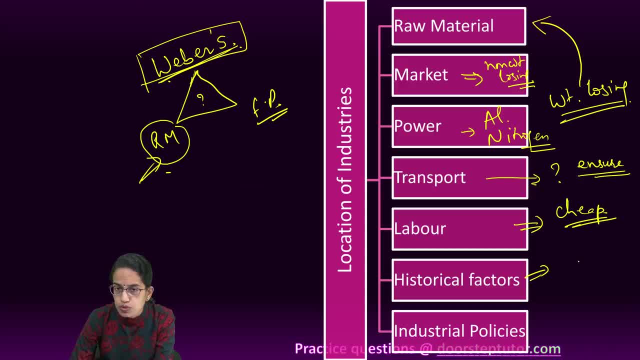 Surat, Vadhoda, Murshidabad, Coimbatore, Kozhikode, Mysore- These were some of the historical areas. Now, during the phase of colonialism, these were the areas where rapid expansion started. 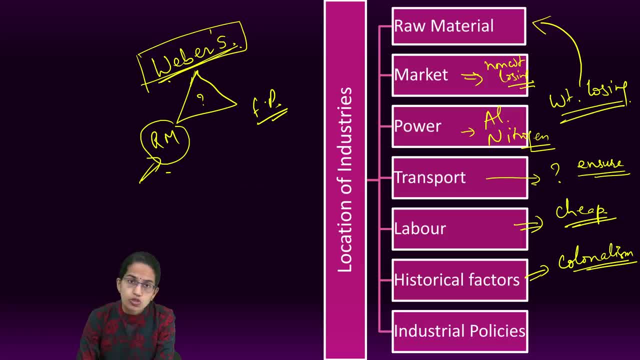 And this also led to discriminatory policies during the colonial time, which eventually led to establishment and more industries which could flourish in those areas. The next is industrial policy, For example, establishment of plants and agricultural products like Billa Bilai, Rahul Kela. These were the decisions to strengthen the tribal pockets in India. 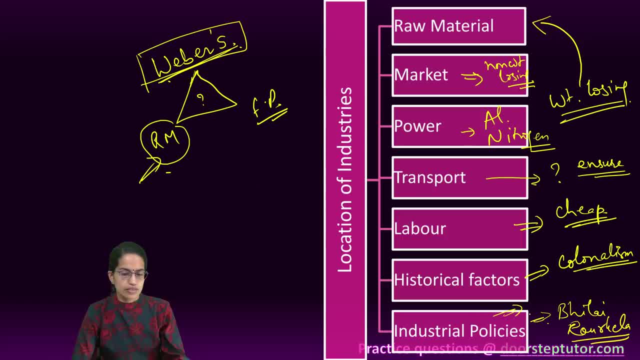 And the government's incentive to provide support to the tribal regions was an idea through the various industrial policies. So industrial policy definitely is an important factor in localization of industry. Now the classification of industry and factors affecting the localization of industries are extremely important for the development of a developed industry. The classification of industry. 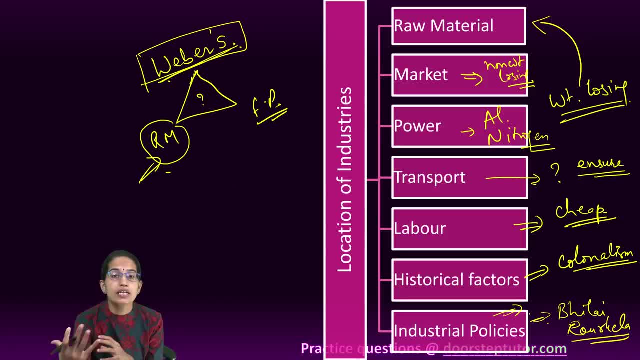 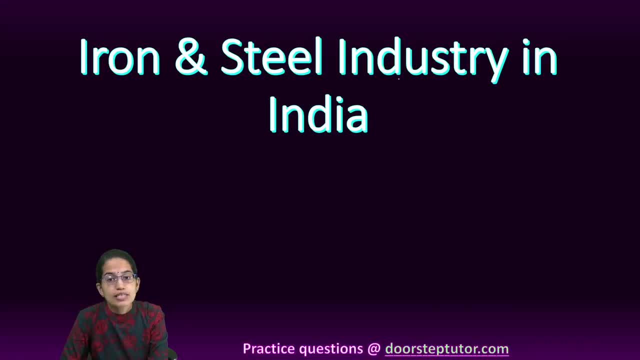 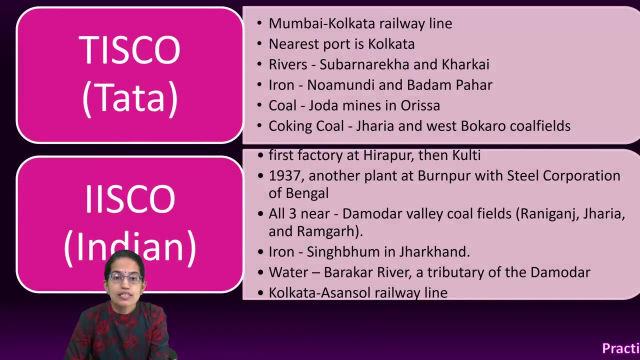 for us to understand before we proceed with the individual industries in all means. One of the most important industries in India is the iron and steel industry, which is called as the pillar or the foundation of industries. Now, iron and steel industry requires what? 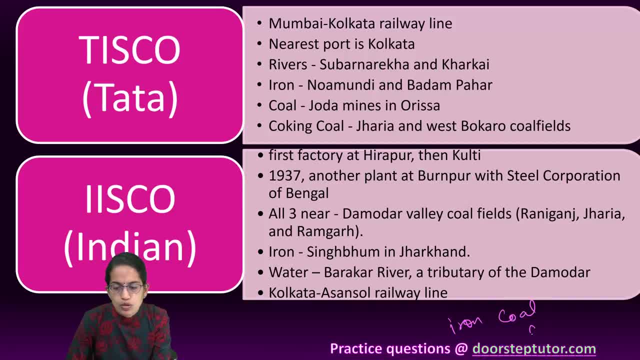 As we know, iron is required. We have coal, coking coal- Then there are limestone requirements, dolomite requirement, manganese and fire clay. So limestone, dolomite, manganese and fire clay are some of the things which are required in the processing of iron and steel industry. 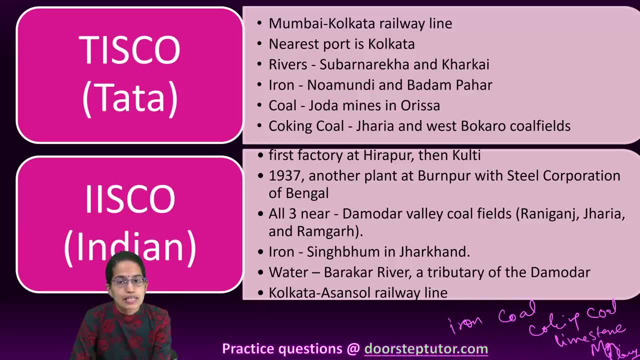 Now, as we mentioned before, iron and steel is a weight losing industry. That means what happens is these industries have to be located close to the source of iron and coal, Because in the process of transportation a lot of weight would be lost and it would 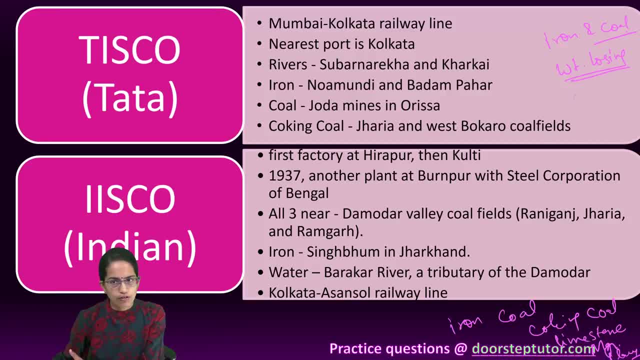 be actually cumbersome to transport the raw material to far off places. So rather than transporting the raw material to far off places, it is a better decision to establish the industries close to the source of raw material. Now we would, in this section, be understanding about some of the major iron and steel plants. 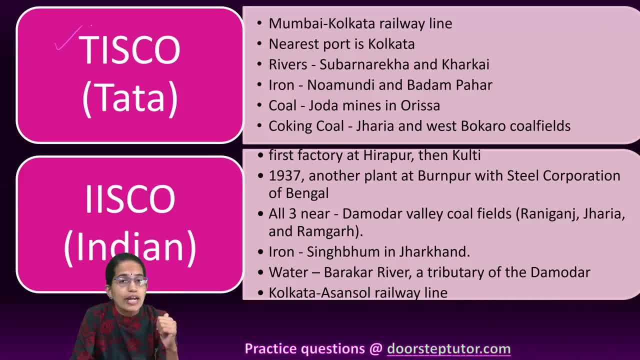 in India. The first that we would understand is technology. Tata Iron and Steel Corporation was the first private establishment of a steel plant in India, and it is located on Mumbai- Kolkata railway line. Now we would understand what are the sources. For iron, it is the Noa Mundi and the Badam Pahad. then we have for coal, the Jodha Mines. 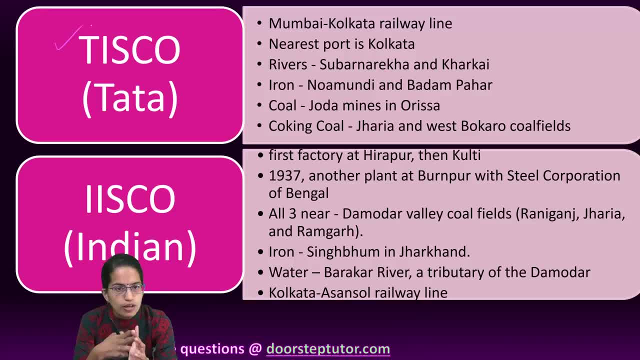 from Odisha, coking coal from Zaria and West Bokaro, and two important rivers flowing here which provide source of energy, And those are Supranekha and Kharkhai. Also, the port for transportation is close by, which is Kolkata, as it is located on the 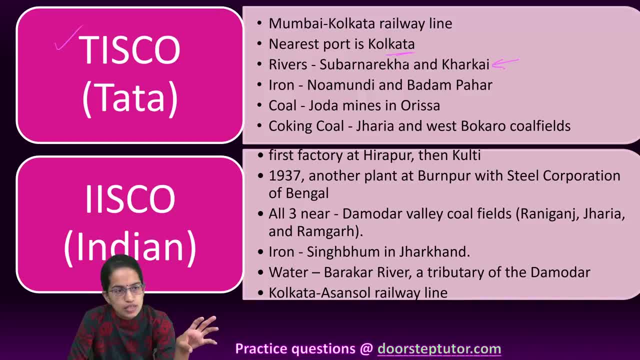 Mumbai- Kolkata railway line. This is one of the best suitable ports which could be transporting the finished product. So this is about TISCO Now. similarly, we have ISCO, Indian Iron Steel Corporation. Now the first factory was established at Hirapur. 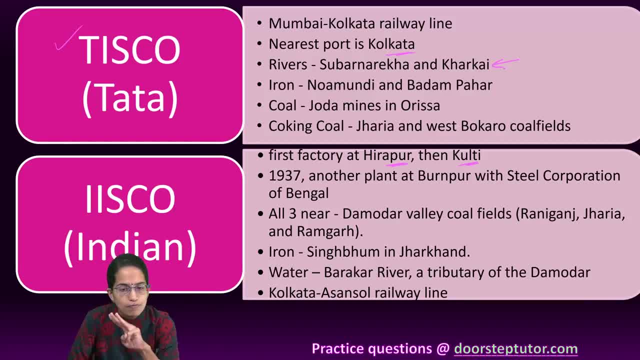 The second factory at Kulti And the third factory at Burnpur. And this third factory, in 1937, was established in cooperation with the Steel Corporation of Bengal. All of these three derived the coal from the Damodar Valley Coal Fields, which is the Ranigan. 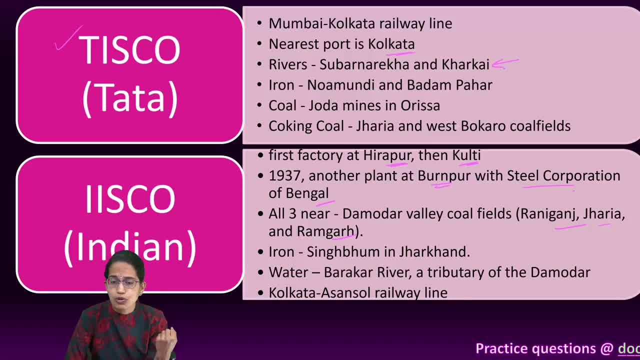 Zaria and Ramgad. So these are the centers from where coal is derived. Iron comes from Singhbhum in Jharkhand. So, as you can see, it's not just one region, it is the nearby areas which also provide. 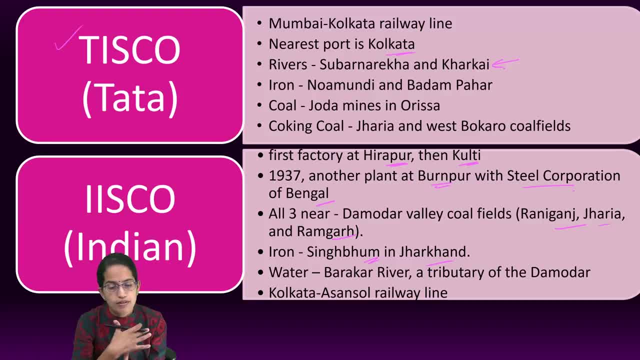 the raw material Water comes from Barkar River, which is again a tributary of Damodar River, and this lies on the Kolkata-Asansol railway line. Now, steel production significantly declined in 1972-73 when this plant was taken over. 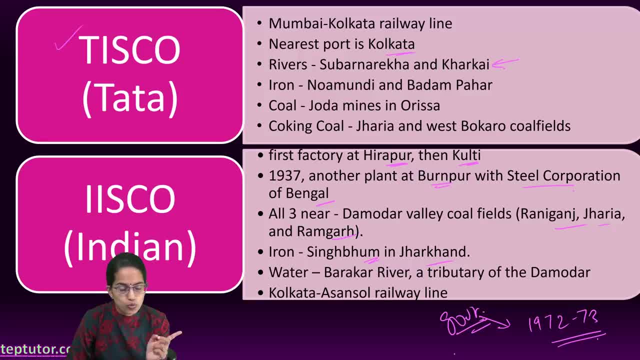 by the government. Now this was one of the reasons where the production from ISCO significantly declined. So TISCO and ISCO again. we have talked about the sources for coal Iron, the major rivers flowing through these areas, the nearby ports and the railway line. 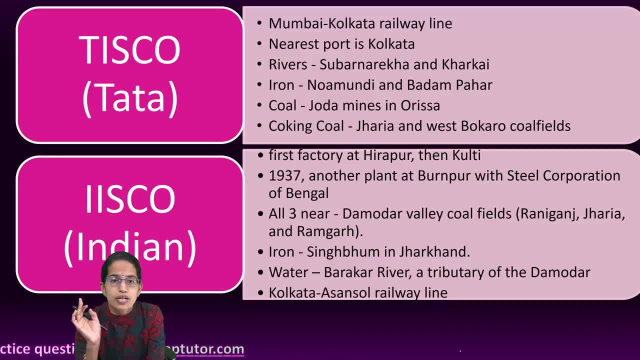 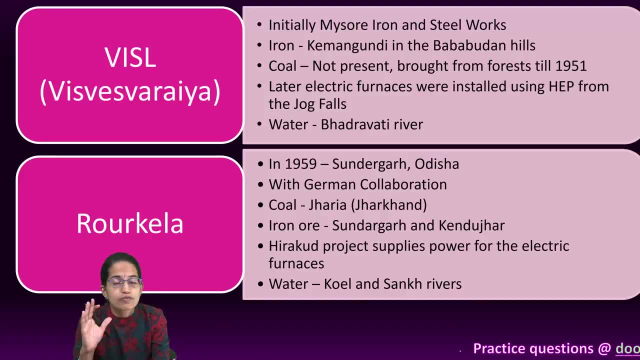 on which they are located. All of these are extremely important information that you have to memorize no other ways, but they are exceptionally important. The next is VISL Vishwishwariya Iron and Steel Limited. Now, Vishwishwariya was initially known as Mysore Iron and Steel Works. 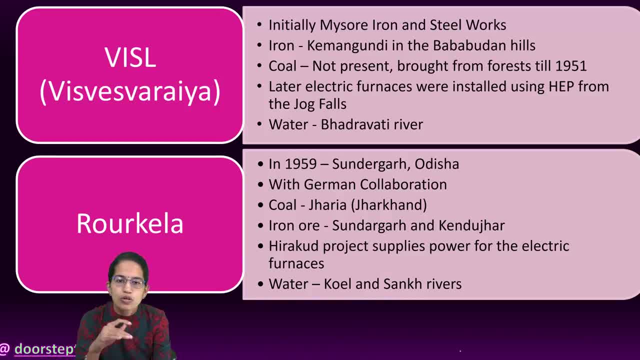 Now, iron came from Keman Guddi in the Babubudin Hills. Coal was not present in the region, But it was brought from the forest, So iron came from Keman Guddi in the Babubudin Hills. 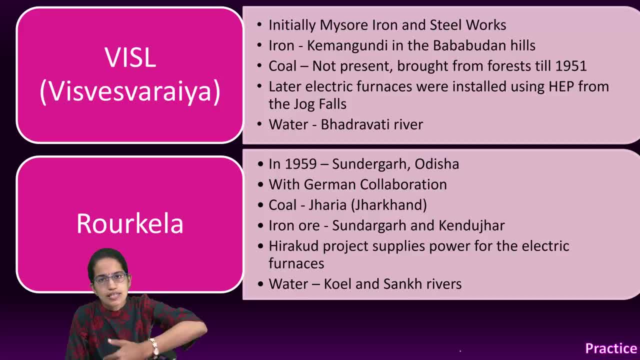 Coal was not present in the region, But it was brought from Keman Guddi in the forest till 1951.. However, later, rather than coal, electric furnace was established and for electric furnace water was used from Jock Falls. 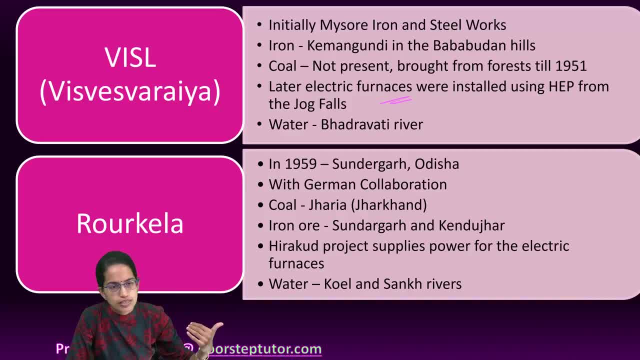 So Jock Falls was the source of hydroelectric power to the project and water from Bhadravati river. Now this Vishwishwariya specializes specifically in steel and specialized alloys and therefore is a very, very important plant. The next important plants that we would understand are iron. 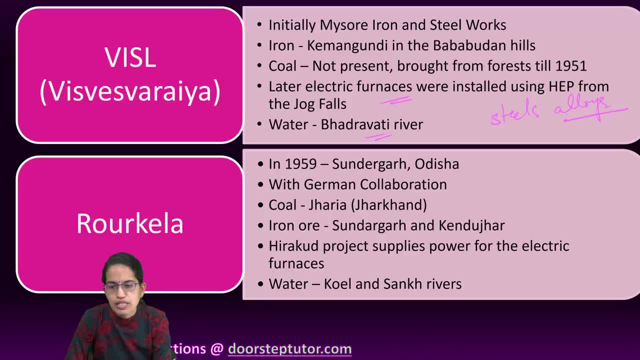 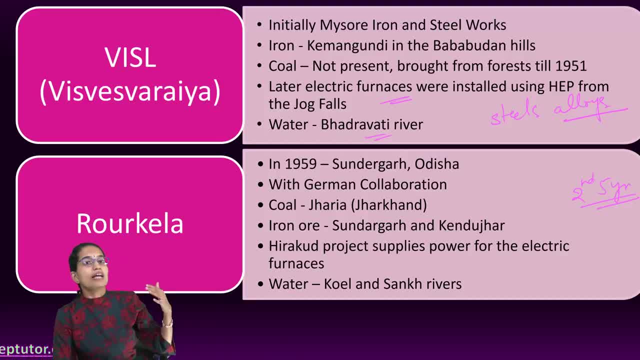 five year plan. So in India we had the five year plans which were released. Now these five year plans, the aim was to develop country on a systematic flow. During the second five year plan, the idea was to have integrated steel plants in India. 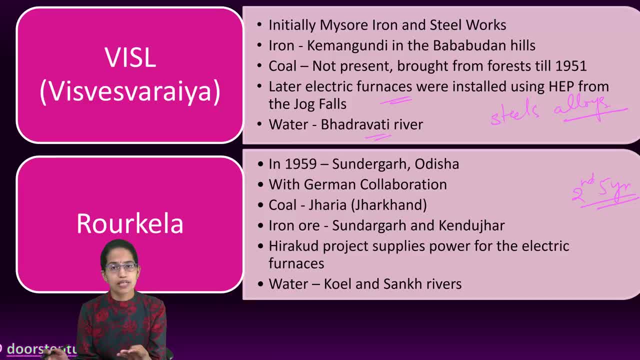 and three important steel plants came in India with different collaborations, So they were in collaboration with different nations expenses. to know about different steel plants- extremely important questions asked often. In 1973, SAIL, which is the Steel Authority of India Limited, was also established in order to manage these plants. So among these, which is Rahul Kela. 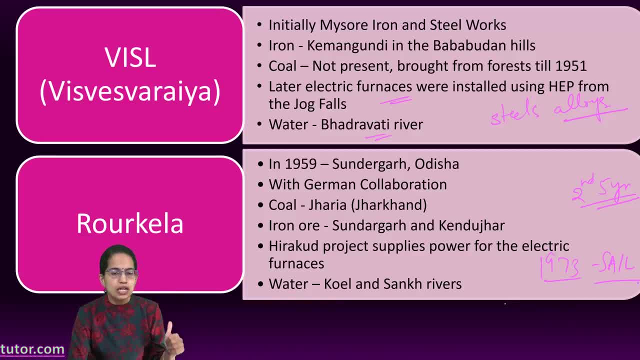 Bilai in Durgapur. Let's understand Rahul Kela first. Rahul Kela was established in Sundargarh in Odisha in 1959 and this came with German collaboration. So Rahul Kela came in collaboration with Germany. Coal was obtained from Zaria Mines, iron ore from Sundargarh and Khejundjar. 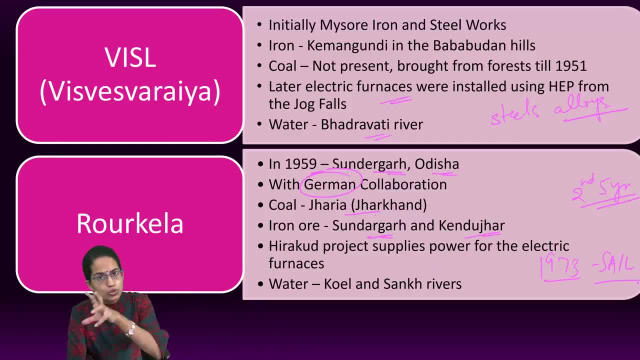 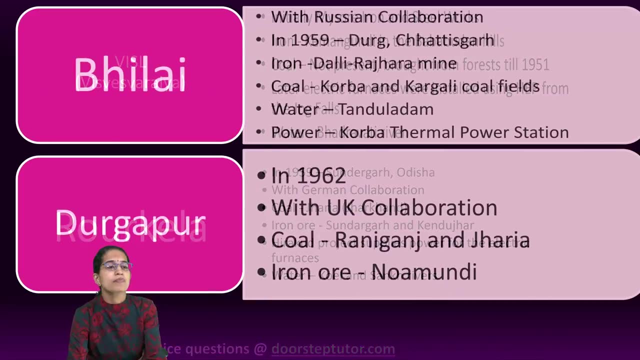 Hirakund power project supplied power to the electric finance in Rahul Kela and water came from Koyol and Sankh rivers. So that was about the Rahul Kela. Rahul Kela, I repeat again, came in collaboration with Germany. Very, very important question. The next is Bilai. Bilai came in with 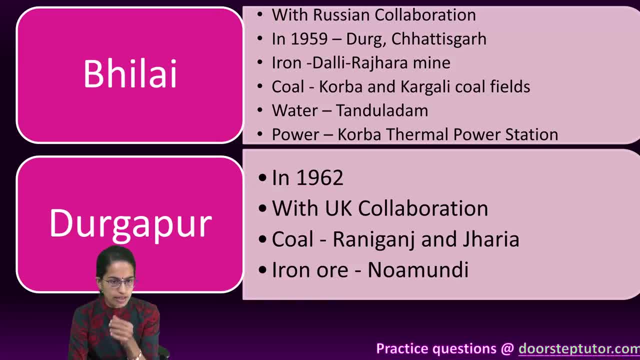 Rahul Kela. Rahul Kela was established in Durgapur. Let's understand Rahul Kela. Rahul Kela was Russian collaboration and Durgapur came in with UK collaboration. So Bilai was established in Durg. So remember Durgapur not in Durg, Bilai in Durg. Okay, So that's just a crisscross that you 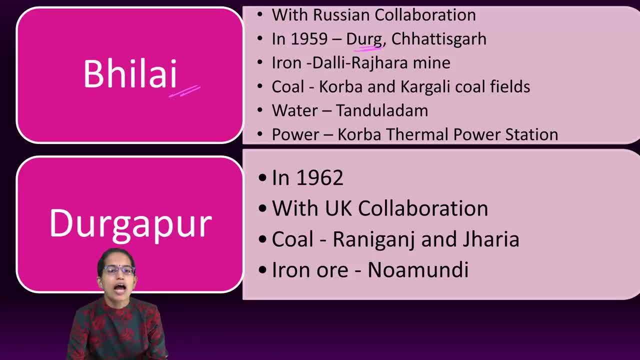 would have to remember. So Bilai was established in Durg and it came with Russian collaboration. So Durg in Chhattisgarh was the location where Bilai. We have iron coming from Dalia Rajahar Mines, Coal from Korba and Kargali Mines, Water from Tandula. 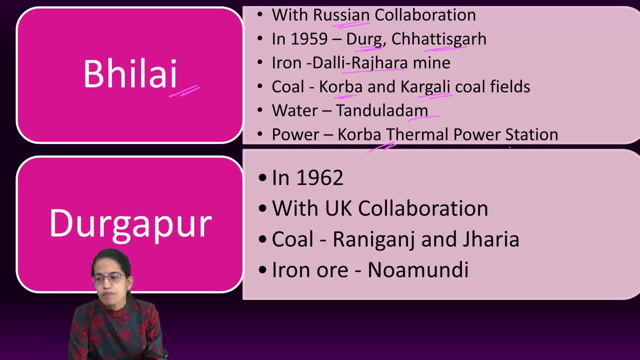 And power from Korba Tharbal plant, Now Bilai plant, lies on Kolkata- Mumbai railway line and most of the steel which is produced here goes to Hindustan shipyards through Vishakapatnam. So again important for you to remember. The next is Durgapur. Durgapur came in 1962 during the 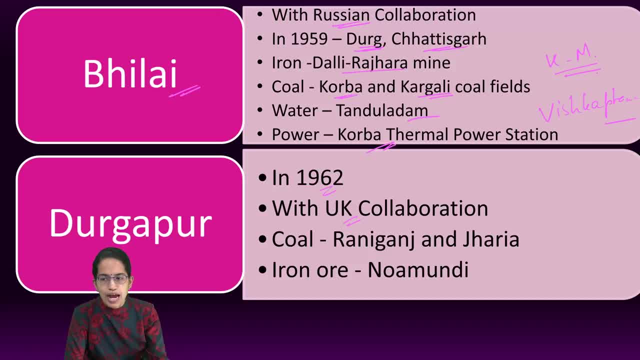 second five-year plan with collaboration of UK, And here we had coal from Raniganj and Zarya and iron from Noamundi. So this is the second five-year plan And here we had coal from Raniganj and Zarya and iron from Noamundi. 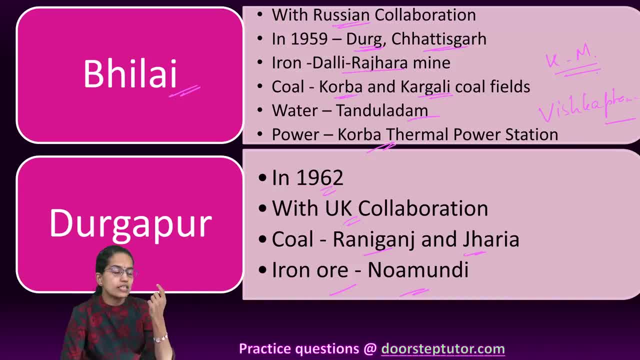 And here we had coal from Raniganj and Zarya and iron from Noamundi. And here we had coal from Raniganj and Zarya and iron from Noamundi, Similar to the iron which was obtained in Tisco. Now Durgapur is important and it is on Kolkata. 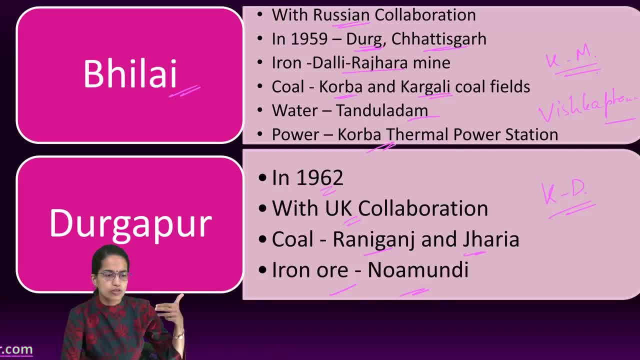 Delhi railway line, So Bilai on Kolkata Mumbai railway line, Durgapur on Kolkata Delhi railway line, And power is obtained from Damodar Valley Corporation, or DVC as it is called as Now. this was not just the end. In South India, we had numerous steel plants which were established. 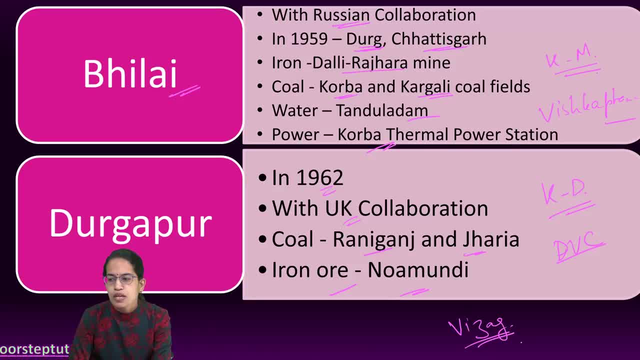 So Vizag plant, which is in Vishakapatnam, Was established and this was an important plant. It was based in Andhra Pradesh And this was the first port based plant, So it was based on the port area, So port based plant and it started. 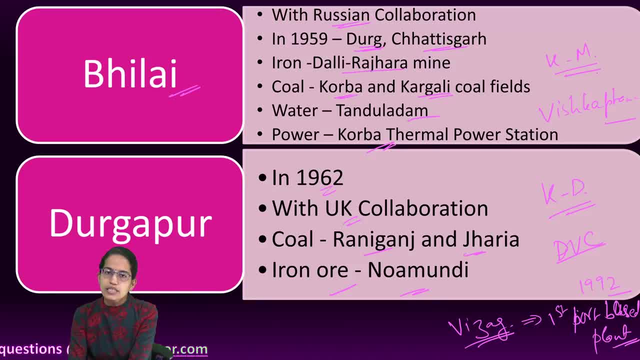 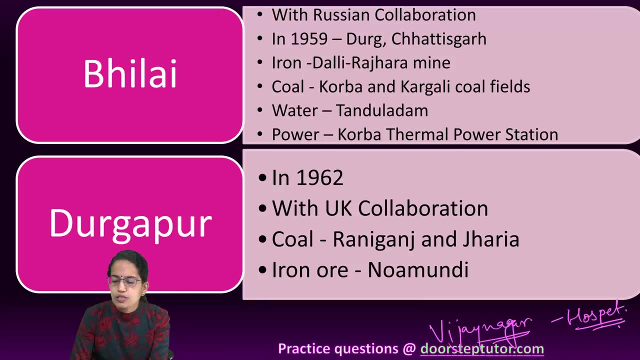 its operation in 1992.. The port location gave it a extreme important advantage. The next was the Vijayanagara steel. Vijayanagara steel plant was another important plant which was established in the Hospit region in Karnataka, And this was developed based on indigenously built technology. 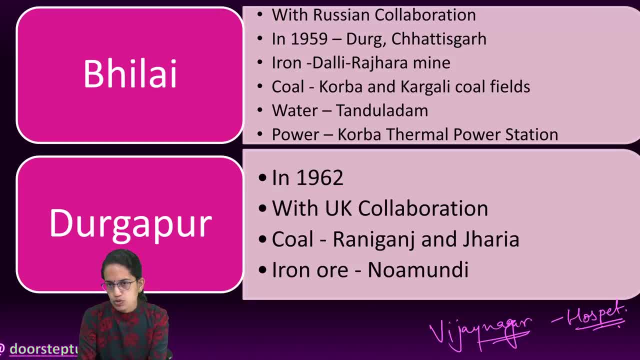 and therefore important. It used locally the limestone and iron ore which was present there. The next important plant is the Salem plant. Salem plant, again in South India, in Tamil Nadu, was commissioned in 1982. So three important plants in South India: Vizag, Vijayanagara and Salem. 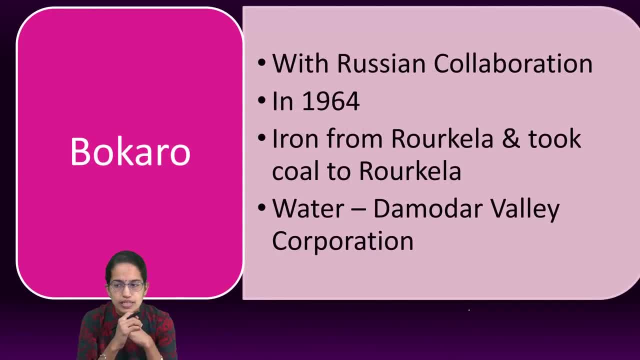 The next important plant that we understand is the Bokaro steel plant. Again, Bokaro, similar to Bilai, came with Russian collaboration in 1964.. Iron was obtained from Rahul Kela. The most interesting thing is Bokaro and Rahul Kela had close ties. 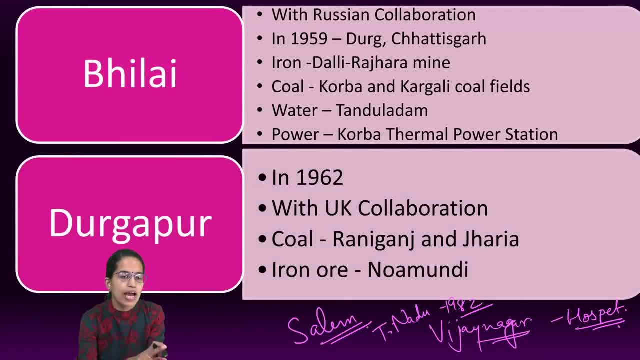 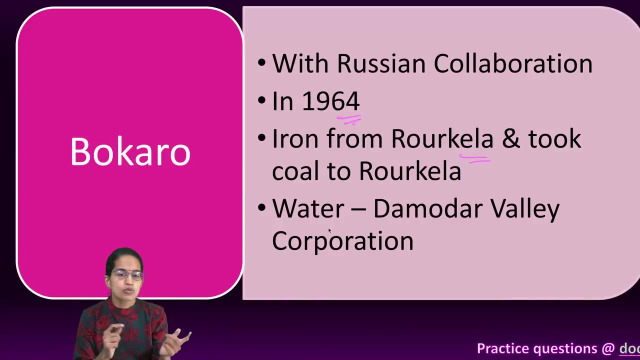 because in the region of Rahul Kela we had the transportation of the coal from Zaria And here in Bokaro the iron was brought from Rahul Kela And Rahul Kela required coal, So that coal was taken from Bokaro to Rahul Kela. So it was actually 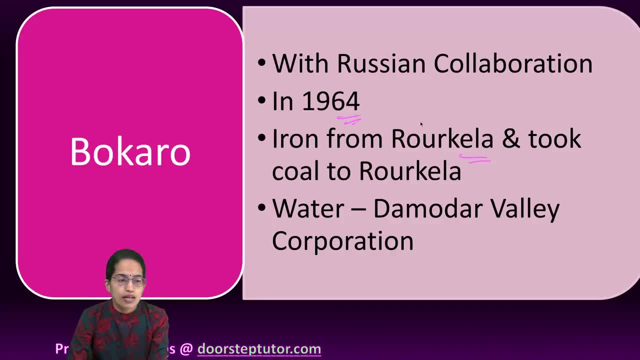 satisfying the needs of both the plants, And this plant utilized water, again from the Amudar Valley Corporation. The most important thing was that a common route was built, which was known as Bokaro- Rahul Kela route combined, And this was where most of the transportation was done Initially. these 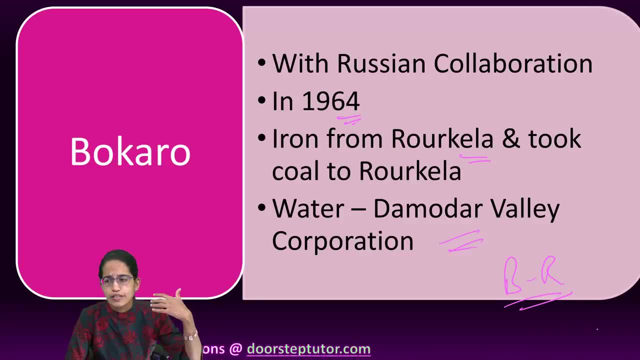 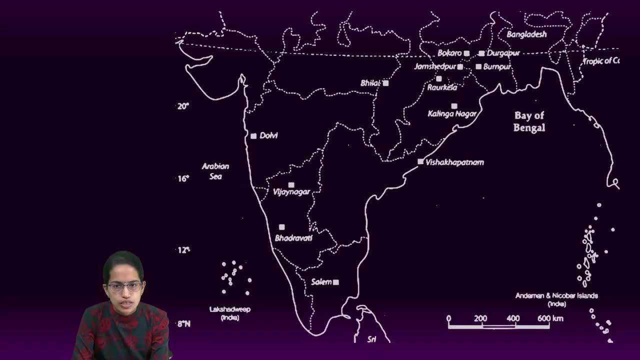 were the major plants which were established, But over the times we had numerous applications, Other small units and more than 200 units were established. Also, most of them use scrap iron as a raw material for manufacturing and in the process of electric finance. So here we have the location and, as you can see in this map, Bokaro, Jamshedpur, Rahul Kela, Burnpur, Durgapur, Bilai are some of the locations which are located very, very in proximity, closer to the source of raw material and the major rivers flowing through there. However, in south we had Selon Beror. 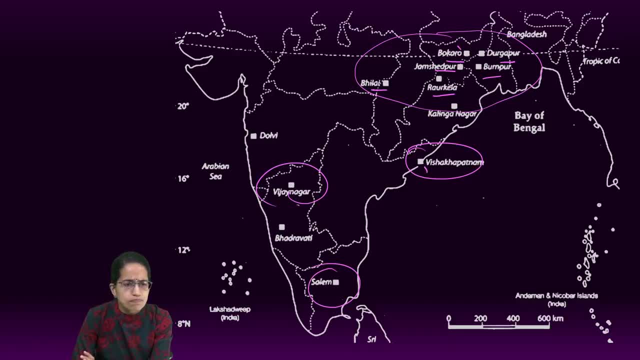 Vijayanagar, Vizag or Vishakapatnam plant. We also had Padravati steel plant, which is another important plant. So those are some of the steel plants and the important major steel plants in India. The iron, the source of iron, the source of coal, the major rivers flowing through these. 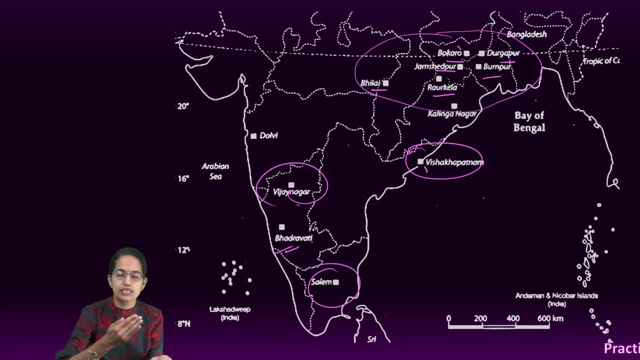 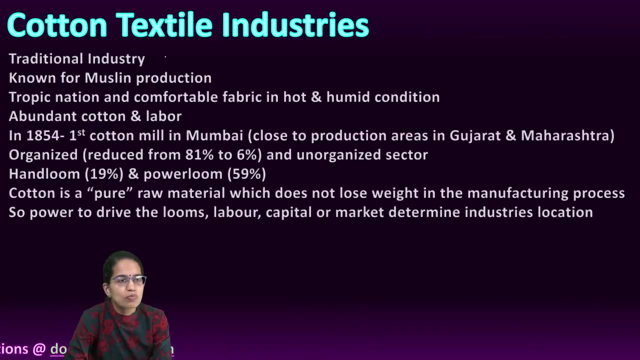 major steel plants are extremely important, and which steel plant came in collaboration with which nation is again an extremely important question. So in the next sections we would cover other major industries in India. The next industry is cotton textile industry. It's one of the most 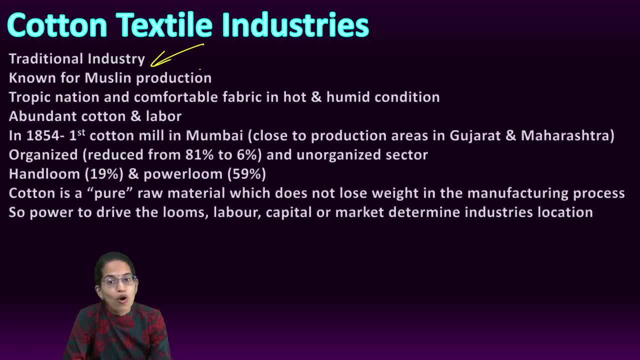 traditional industry and India originally, is known for muslin production. The quality of the cotton which we have is extremely known. Again, the climate is one of the major factors, because the Indian climate is predominantly a tropical climate and therefore cotton fabric provides comfort in hot and humid conditions. So cotton was in demand since long. 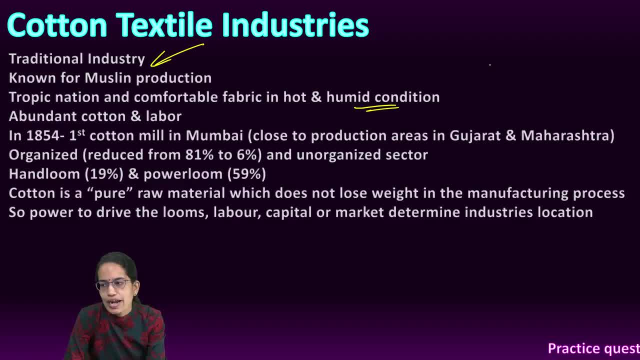 Now, initially, what happened? We do had our indigenous cotton textile technology, but with the advent of Britishers, the cotton started to move to Britain and therefore we had the finished product, which landed back in India. Despite the fact we had abandoned cotton and labour, most of our mills were not established in India. 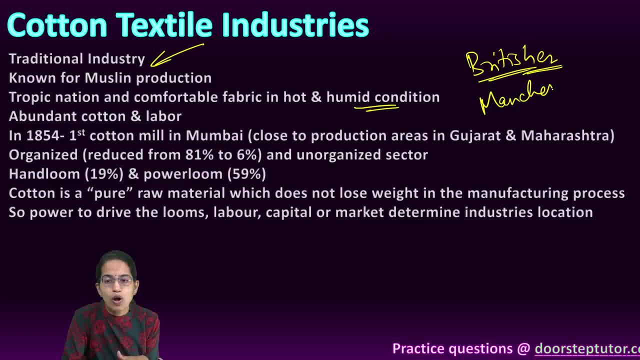 And from Manchester and Liverpool the product was brought back to India for for sale. Now, this was some of the things which led to a factory revolution, or what we call as industrial revolution, in United Kingdom, because there was mass production of the textile there. but, however, in 1854 we realized that 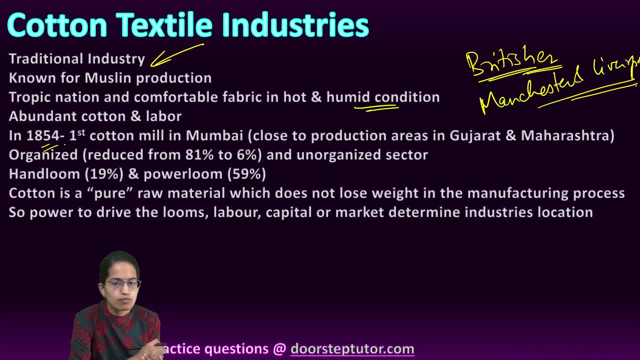 India should have its own cotton mill, and the first cotton mill was established in Mumbai. Now, why Mumbai? again, a good question. Because there was cheap labor, Machinery was imported from England and since Mumbai was a port area, the machinery could easily reach the Mumbai. 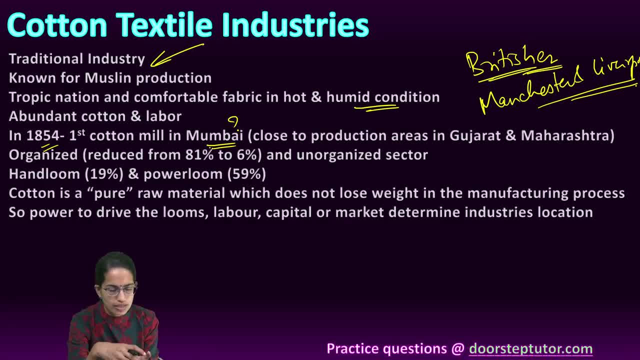 There were good production areas in Gujarat and Maharashtra. Again, if we talk about some of the statistics, during the time of independence there were just few mills in India, which increased to 423 mills after the partition. but during the India faced a lot of good quality growing areas which were there went to West Pakistan. 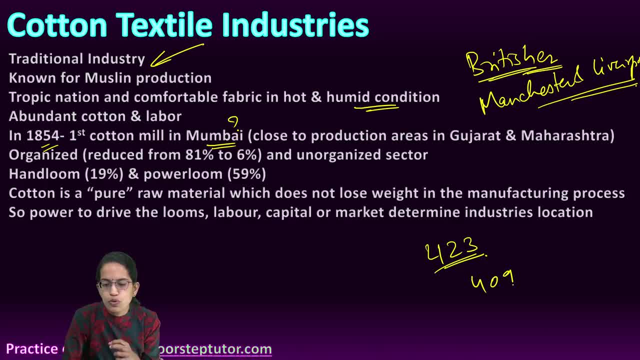 and therefore India was left with just few mills. and few mills had to move to the region of Pakistan. but despite the fact that India had good mills, the cotton producing area which was left with India was only 29 percent. most of the cotton producing area went to the West Pakistan after. 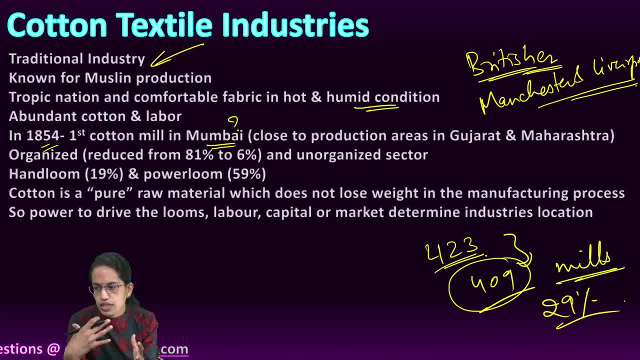 independence, we started to revive and eventually it flourished. in 1998 we had nearly 1782 mills in India, of which 192 mills were in public sector, 151 in cooperative sector and the remaining highest number of mills were in private sector. now again, cotton textile was both in the organized and 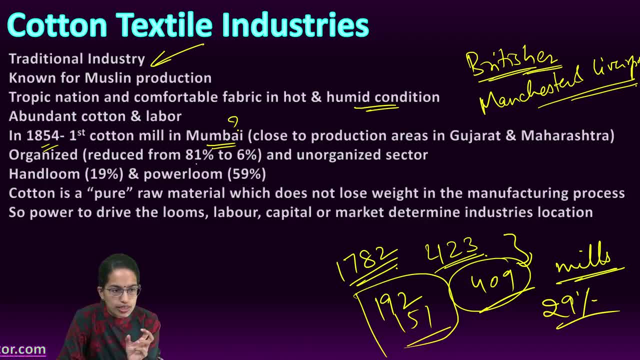 unorganized sector. however, the organized cotton textile reduced from 81 percent to 6 percent. handloom and and power looms were again the major differentiation. however, we were squeezed with the handloom production, which was only 19 percent and most of it was based on power loom. now, as we said, 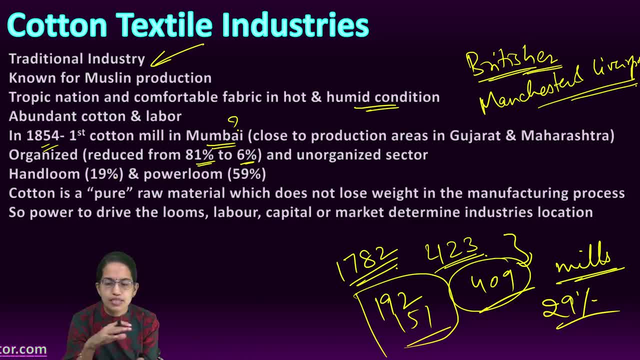 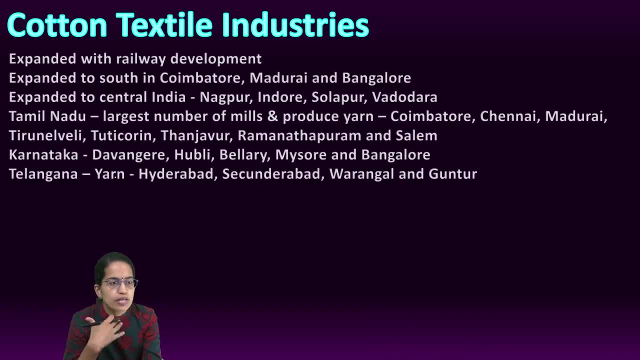 cotton is a pure raw material. that means it does not lose weight in the process of manufacturing. that means cotton could be located close to either labor, either capital, either market. so we would have to decide where the cotton would actually be located. so there were numerous developments and expansion is started. cotton textile mills were established in different 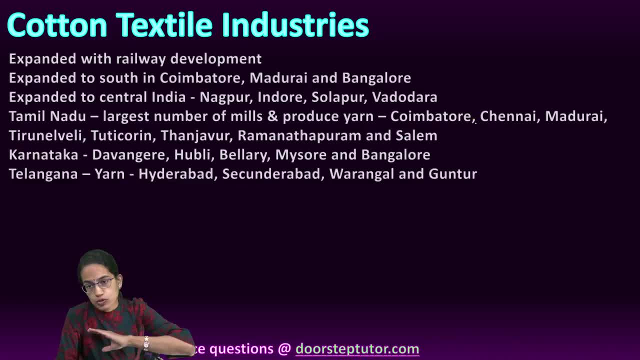 parts of India based on different criteria. there was expansion with real speal line. in the South they were new cotton textiles, So I thought I might get in more detail on the lead up to this. I forgot to mention in release that cotton textiles comes in a box form, semi from this age, one to be分 20 to 나는. 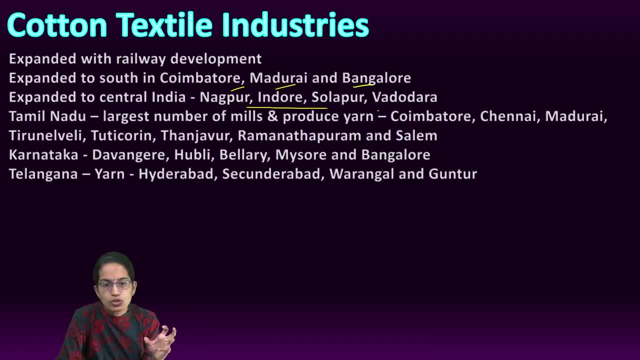 of Coimbatore, Madura I, bangalore in central India post. not curious Colap parenting the other in Gujarat, in the South. the largest number of mills were seen in Tamil Nadu and it manufactures yarn, not the cotton textile he are coming to China's technologies to be used for to 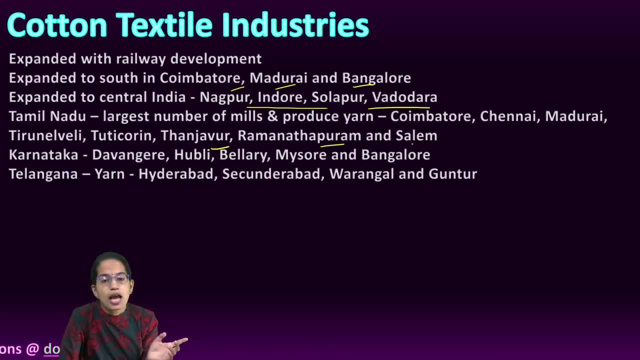 Chennai, Madurai, Tuticorny, Thanjavur, Ramanathpuram and Salem were some of the major centers. In Karnataka- Hubli, Billari, Devangir- and in Telangana again, it was mainly the Yand which was produced. 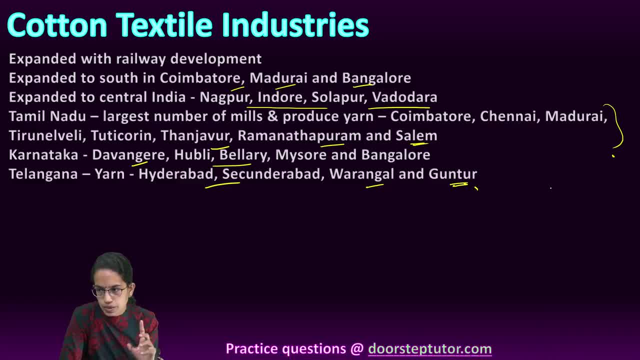 Hyderabad, Sikandarabad, Warangal and Guntur were the areas where it was produced. Now, what was the reason for the localization? For example, Kanpur was the area where cotton textile came because of the local investment. Mills were established in the regions of Kolkata and that was due to the hydroelectric power potential and the port facility which was available. 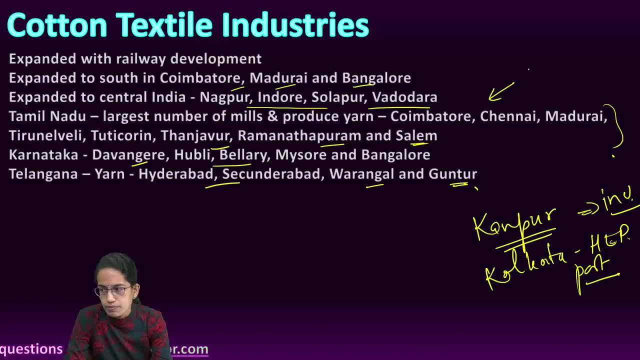 Tamil Nadu, as we know, had abundant amount of water power or hydel power, which was required for the mills, and therefore numerous plants for cotton textile were established in the regions of Tamil Nadu. Similarly, we had various regions where different regions, regions- were responsible for establishment of cotton textile industry. 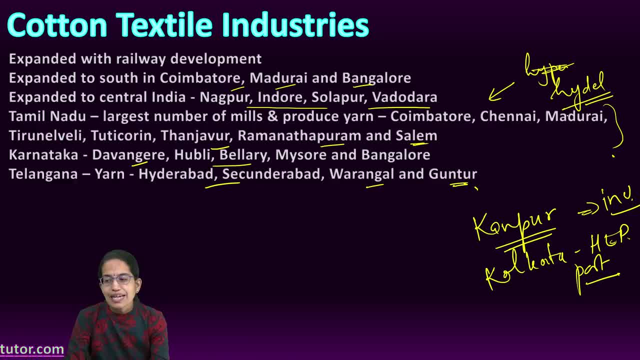 In Uttar Pradesh, Kanpur became one of the major centers. Besides Kanpur, Hathras, Saharanpur, Modinagar, Agra, Lucknow were other major centers. In West Bengal it was predominantly the Hugli area. 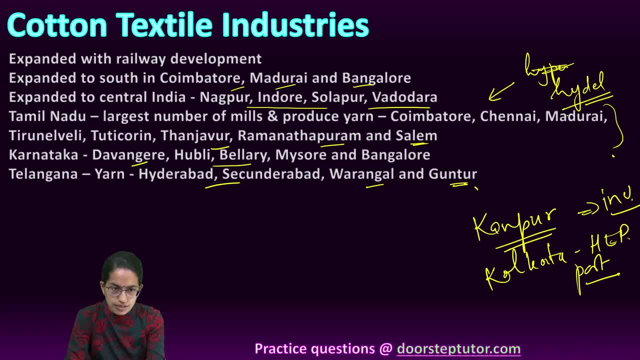 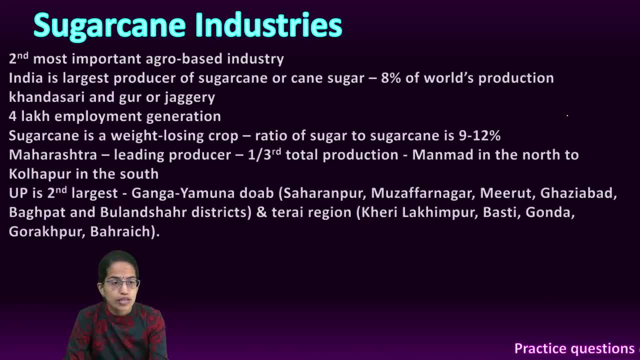 Then Havra, Serampur, Kolkata, Shyamnagar were some other important areas. The next important industry was the sugarcane industry. Sugarcane was the second most agro-based important industry, and it not just produces sugar. 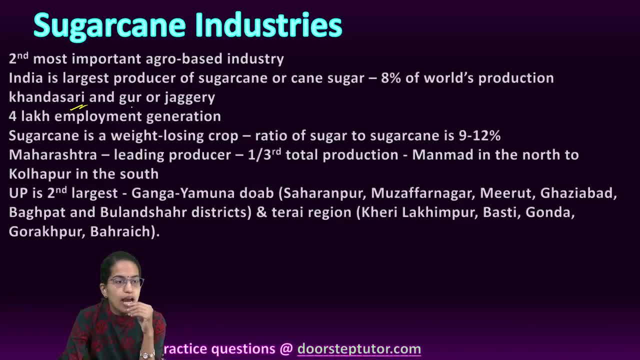 sugarcane was the second most agro-based important industry, and it not just produces sugar, but it also produces Khansari and gur, which is jaggery. Now India in the world is the largest producer of sugarcane, as well as cane sugar. 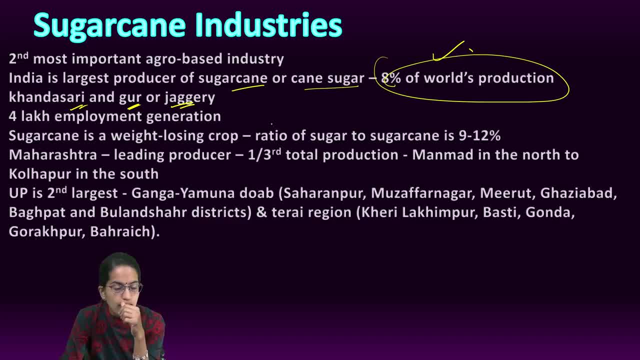 8% of the total world production comes from india and it provides employment to 4 lakh people. Now, sugarcane is a weight losing industry. That means the industry has to be located close to the source of raw material. now the ratio of sugar to sugarcane is 9 to 12 percent. 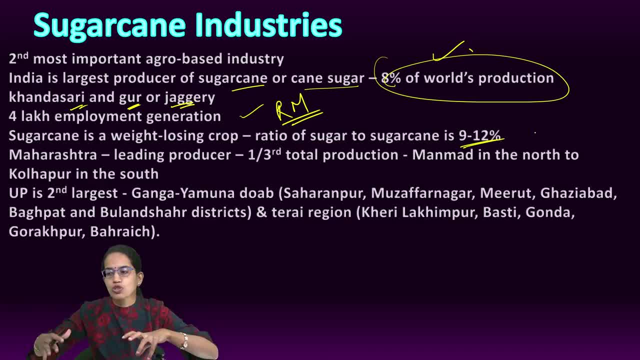 Now the ratio of sugar to sugarcane is 9 to 12 percent. That means the sucrose content begins to dry up after it is harvested. So if it is immediately consumed within 24 hours of harvesting, best recovery of sugar can be witnessed. 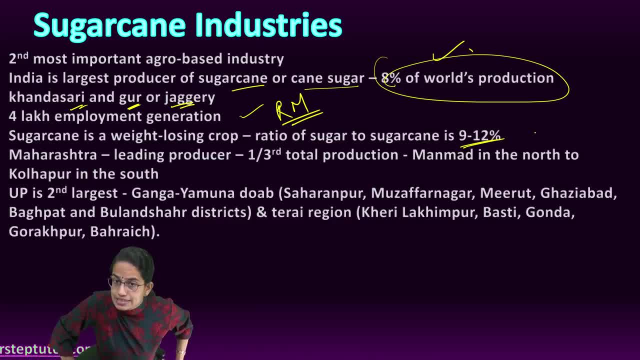 Based on this, the sugar industry, which is mainly a seasonal industry we have seen the highest production comes from Maharashtra, which has one third of the total production. From Manmad in the north to Kholapur in the south is the belt where you have the sugar cane production and the sugar cane industries. 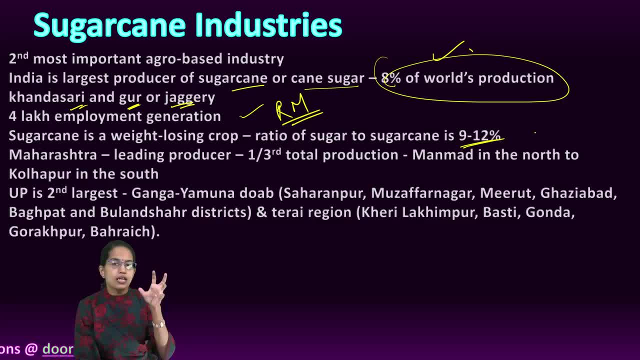 UP is the second largest area. In UP there are two regions: The Gangayamda Duaab area and the Tarai area. In the Duaab area, Saharanpur, Muzaffarnagar, Meerut, Ghaziabad, Baghbat and Bulanshar are the areas. 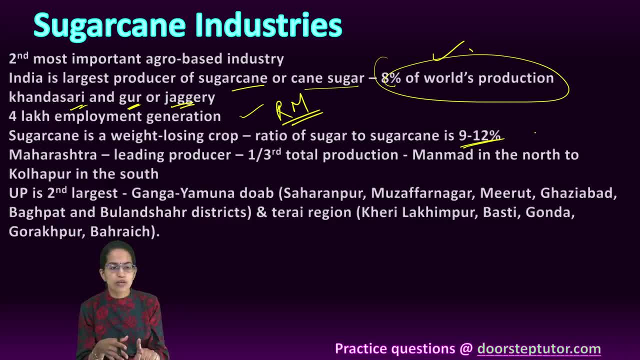 In Tarai area. it is Kheri, Lakhimpur, Basti, Gonda, Gorakhpur and Bharech which are some of the major areas for production of sugar cane. Now, if we look on to the sugar cane industry, 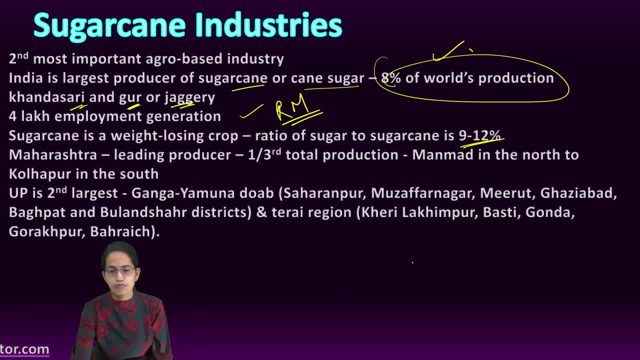 If we look at the development on the model line and date it back to the sugar mill, we see 1903 was the time when the first sugar mill was established in Bihar. Later on you had numerous industries coming up in the regions of Uttar Pradesh. 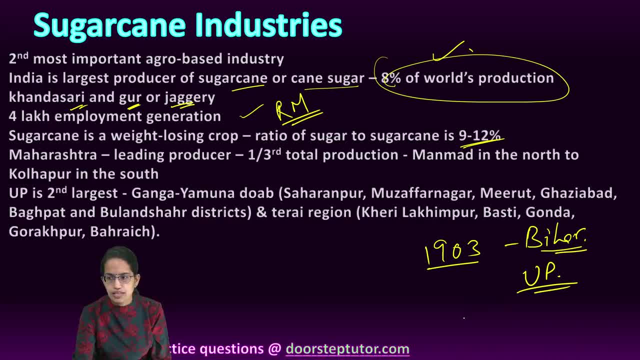 As of now, we have seen a significant increase in the number of sugar factories, from 139 during the time of independence to around 506.. During the independence, there was only just 11.3 lakh tons of production. However, it increased to 17,900, something in terms of production in lakh tons. 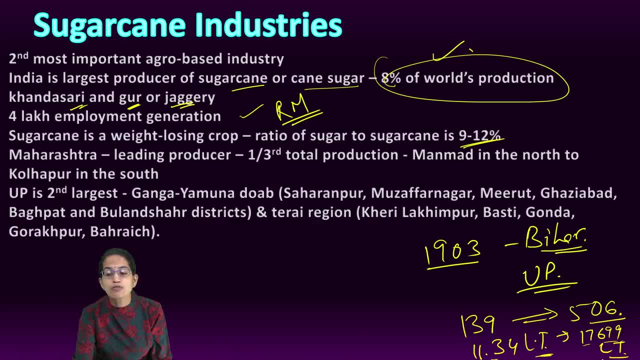 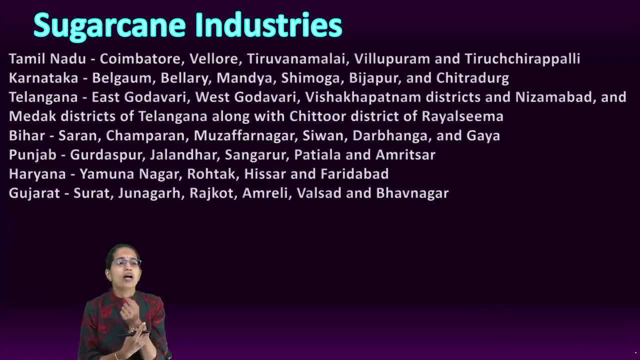 So just from 11 lakh tons it was 17,000 lakh tons. So that was the increase in the production of sugar cane. we witnessed over the years Now various areas and the production. So in Tamil Nadu it is Coimbatore, Vellore, Thiruvannamalai. 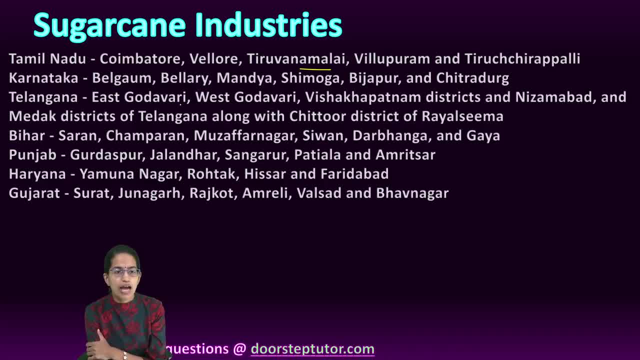 In Kerala it is Belgaon, Bellary, Mandia. In Telangana we have the East and the West Godavari, Vishakapatnam, Nizamabad, Bihar, Saharan, Champaran, Muzaffarnagar. 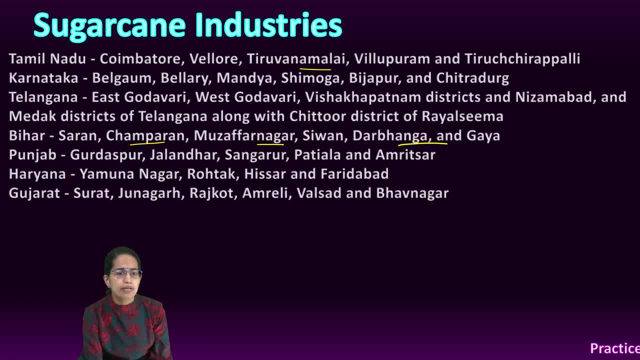 Then we have Darbhanga and Gaya, In Punjab it is Gurdaspur, Jalandhar, Patiala, In Haryana it is Rotakhisar, Faridabad, And in Gujarat it is Surat. 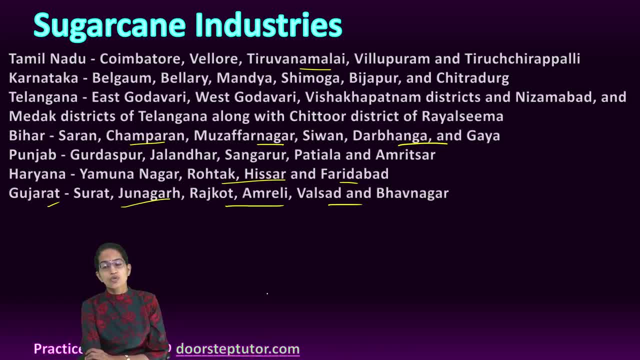 Junagar, Rajkot, Amreli, Vilsad and Bhavnagar. So those are some of the areas where sugar cane industries have been witnessed. Again, the amount of sugar present in the southern varieties and the northern breeds are different. 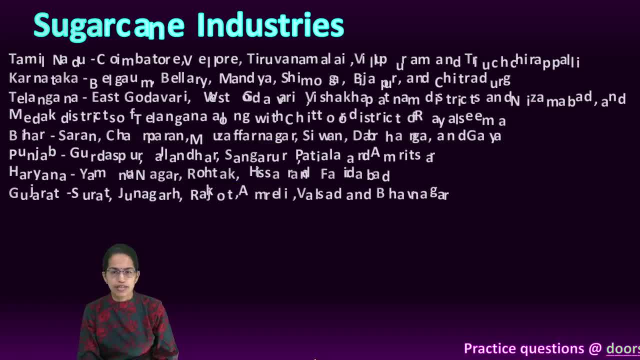 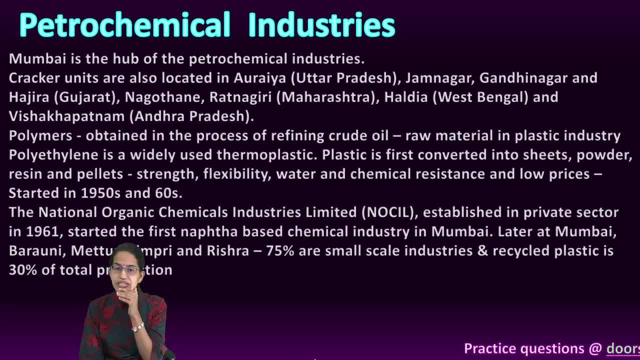 And that's again due to a lot of it is due to the climatic factors. The next important is the petrochemical industry. Now, petrochemical industries are a group of industries which have been growing extremely fast in India. A variety of products come under this category. 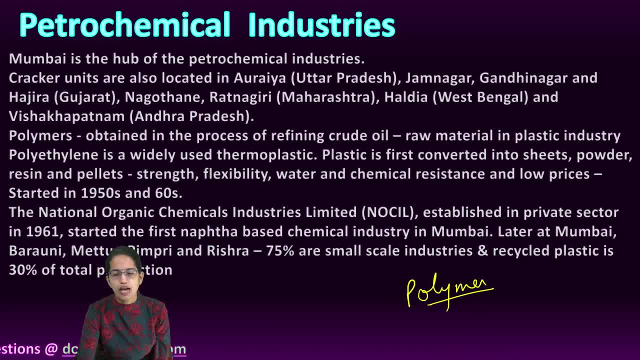 For example, we have polymer. Now these polymers are made by ethylene and propylene. Then we have synthetic fibres, There is elastomers And there are surfactants. So those are some of the common classification for petrochemicals in India. 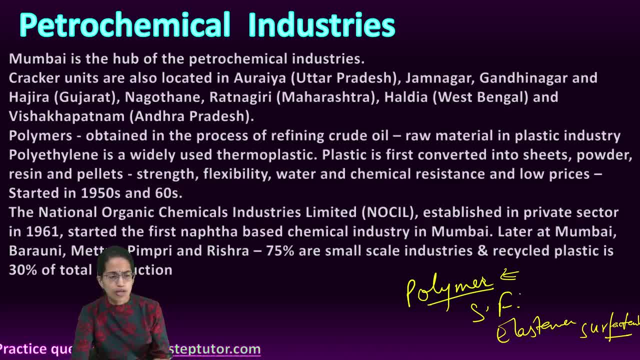 Polymers are predominantly ethylene and polypropylene, And they are used for making plastic. Now, plastic is first converted into sheet powder, resin or pellet, And it is known for its strength, flexibility, durability, resistance and low pricing. 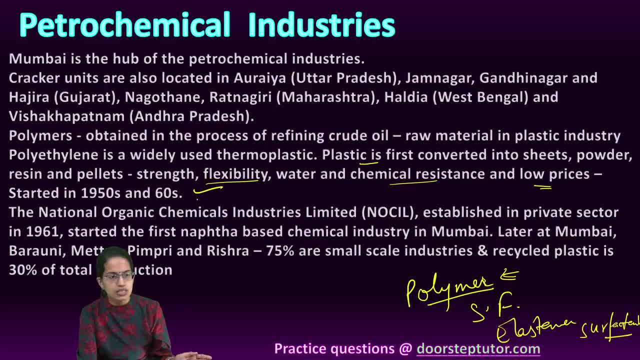 It has started its production in 1950s, 60s And this polymer is obtained in the process of refining of crude oil, And it is also used as a raw material for plastic industry. The National Organic Chemical Industries Limited was established in private sector. 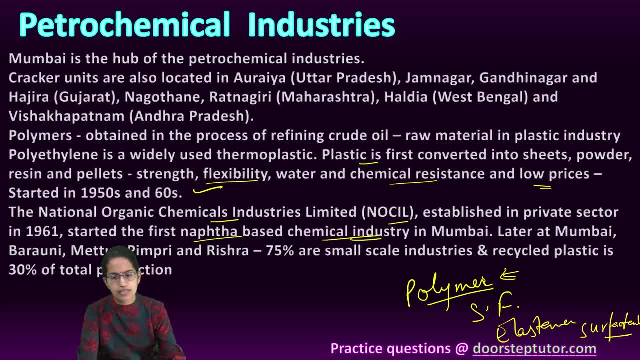 And this was the first naphtha based chemical industry which is started in Mumbai. Later on, Baroni, Pimpari, Rishra were some other industries which were established. 30% of the total production comes from recycled plastic. 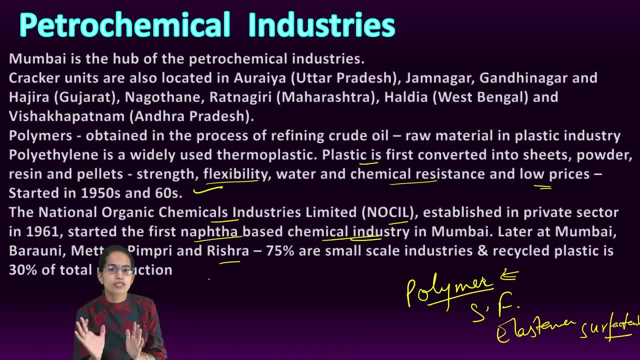 And of the total plastic industry, 75% are small scale industries. Now Mumbai is the hub for all petrochemical industries. Cracker units are seen across India, So in Aurya in Uttar Pradesh, Ratnagiri in Maharashtra. 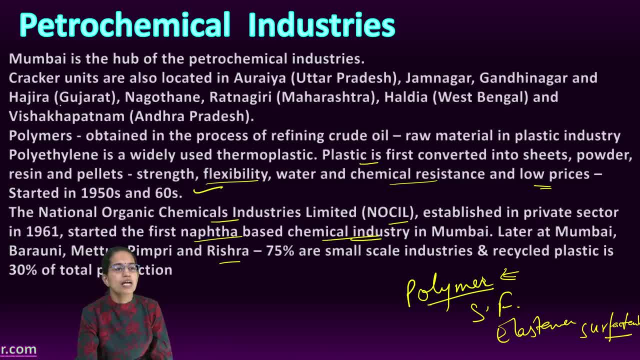 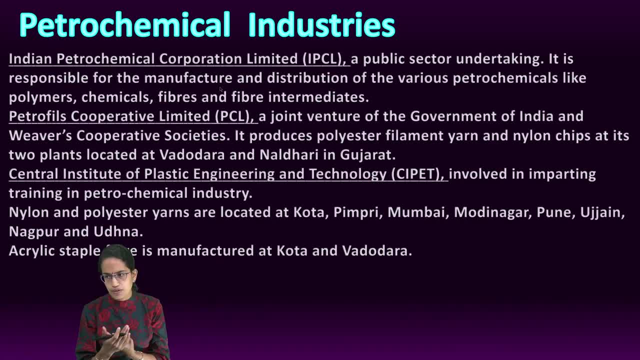 Haldia in West Bengal, Vishakapatnam, Andhra Pradesh, Hazira in Gujarat are some of the common locations where we have the petrochemical industry. The next are the three important organizations which are working under the petrochemical sector. 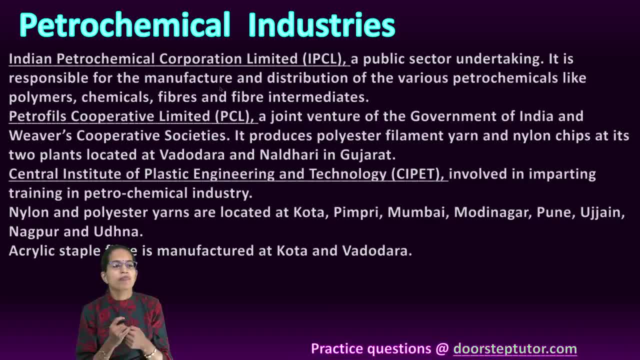 under the department of chemical and petrochemicals. So the first is Indian Petrochemical Cooperation Limited. It is a public sector undertaking for manufacturing of petrochemicals like polymer fiber, fiber intermediates, Petrofil Co-operative Limited, which is a venture of Government of India, and Weaver Co-operative Society. 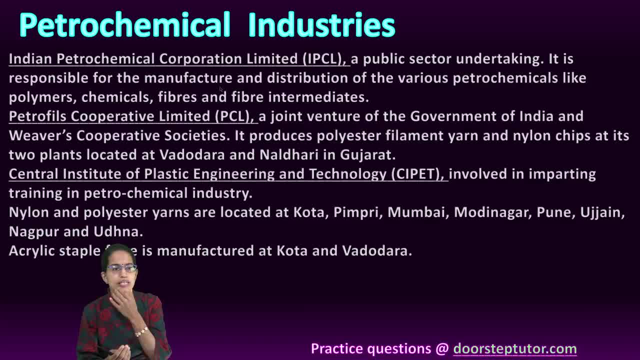 So it produces polyester, palm yarn and nylon chips. It has two plants, which are located in Varodhara and Naldahari in Gujarat. The next is the CSI, CIPET, which is the Central Institute for Plastic Engineering, which imparts training for petrochemical. 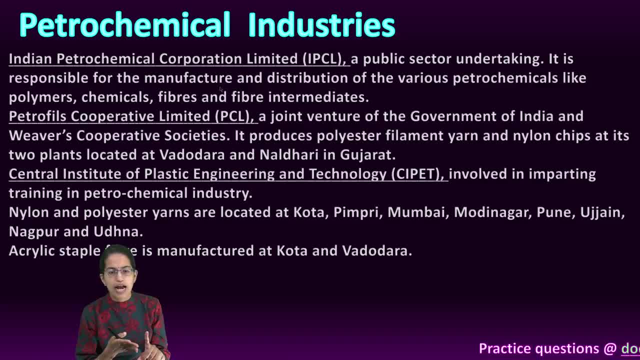 Now, nylon and polyester yarns are made at Kota, Pimpri, Mumbai, Modinagar, Pune and Ujjain. Acrylic staple fiber is made at Kota and Varodhara. So those are some of the important regions where we have the petrochemical industry. 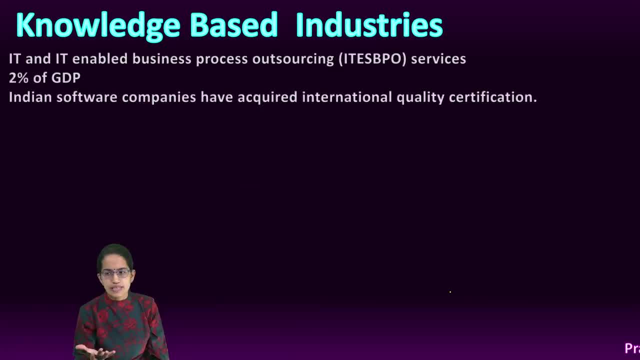 The next is knowledge based industry. Now, knowledge based industry includes the IT industry, which contributes to 2% of the production. It includes the IT and IT-enabled business process, outsourcing, as we call it as ITES, BPO services. So Indian software companies have been known globally for their quality certification. 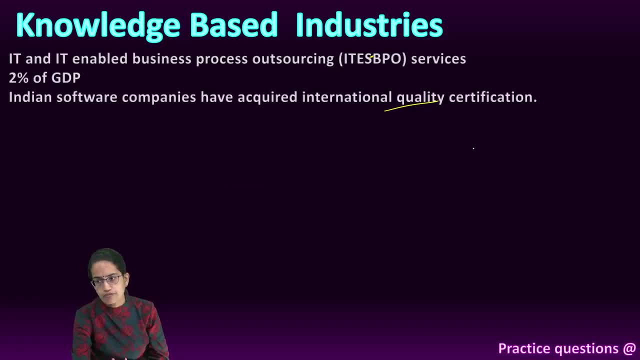 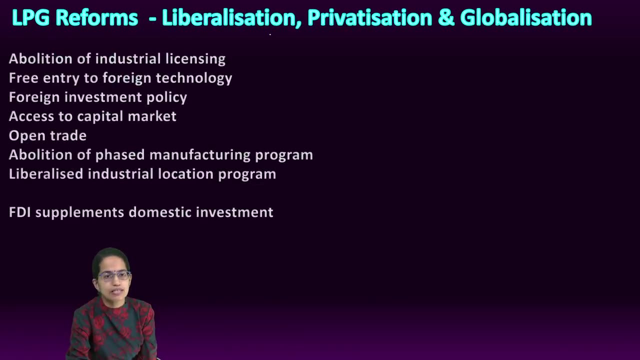 They have surpassed in the terms of electronic hardware production, and government has created numerous software parks across India in order to promote this process. The next important thing is: 1991 was the period of IT. 1991 was the period where we witnessed the LPG reforms, which were liberalization, privatization and globalization. 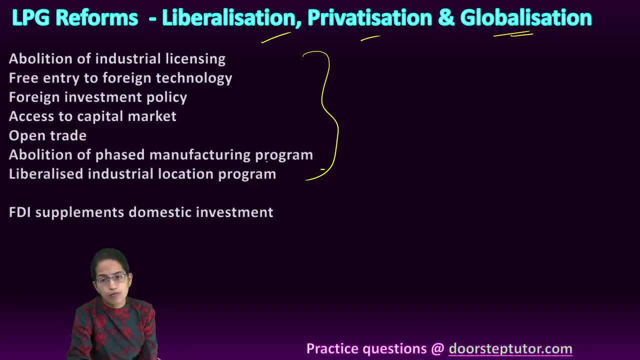 Now when industries are established. these are some of the points which were taken into account: Abolishing the licensing system, free entry of foreign technology, foreign investment to be eased, bringing in access to capital market, open trade, abolishing the manufacturing programs and liberalized industrial location programs. 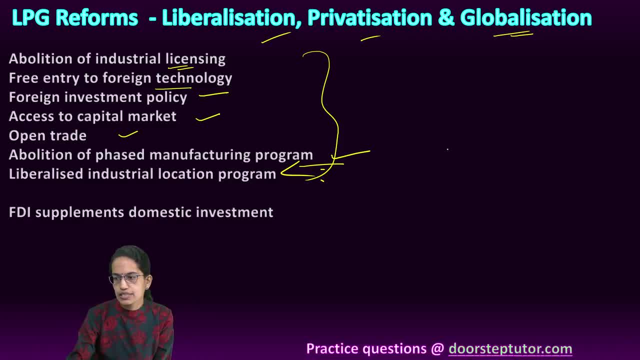 Now FDI supplements the domestic investment, So the licensing system have been abolished for all except the six industries which are related to security, related to strategic purposes and environmental and have environmental concerns. Now, at the same time, the number of industries which are reserved for the public sector since 1956. 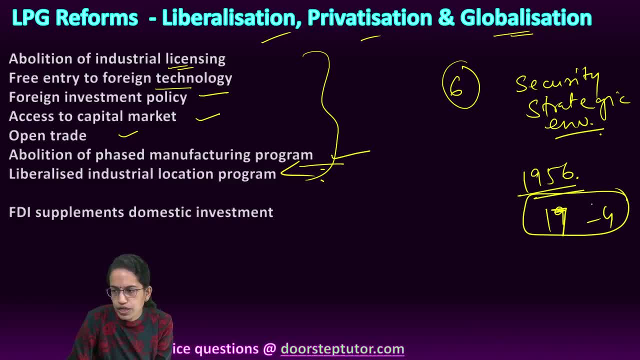 have been reduced from 17 industries to just 4 industries. We have one of the industries which falls under the department of atomic energy. So atomic energy has been in the public sector for the purpose of security. Now FDI- foreign direct investment- is brought into an industry for the purpose of technological upgradation. 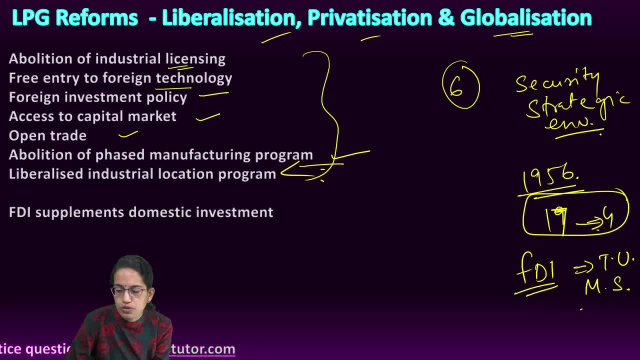 managrial skills which could be developed and good use of human resources and natural resources. So industries are technically discouraged in to be established closer to large cities, existing large cities- because if they are brought closer to the tribal builds there would have more chances of development in those areas which could be witnessed. 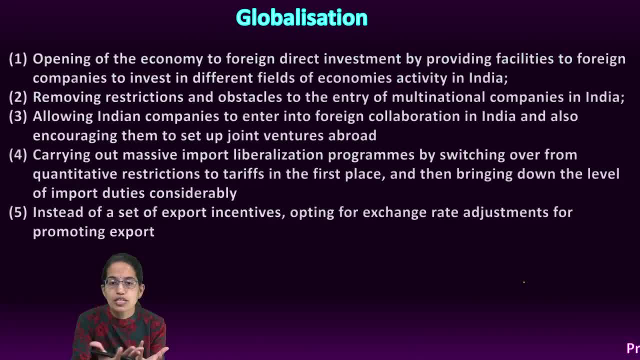 The next is globalization. We say that the world is growing as a global market. So there is integration of economy and integration of the capital, goods, services, labor resources which can move freely from one nation to another. So the idea is open the economy for foreign direct investment, to provide facilities for investment. 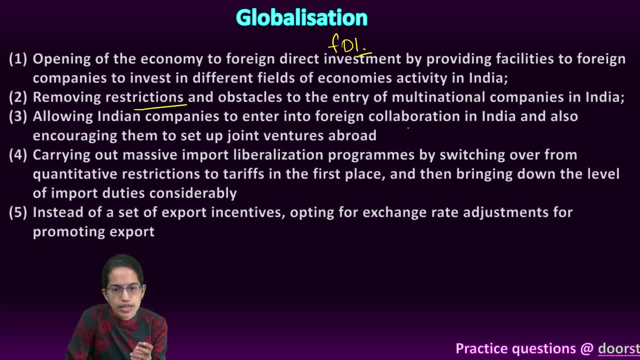 remove the restrictions, allow Indian companies to enter into foreign collaboration, carry out massive import liberalization programs and, rather than export incentives, opt for exchange rate adjustments to promote exports. Now, those are some of the important things that we understand in the process of globalization. 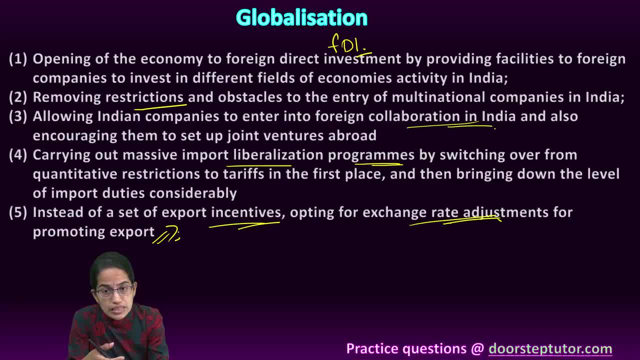 Now in this section we have understood some of the major industries in India and why LPG reform was one of the major reforms in India which paved the way for easy industrial establishments in India, easing the licensing requirements in India, and how globalization opened the doors for foreign direct investment. 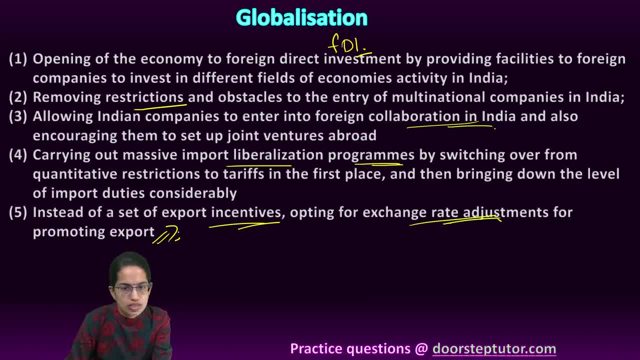 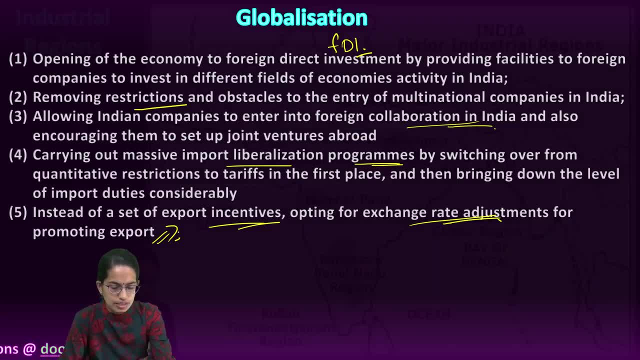 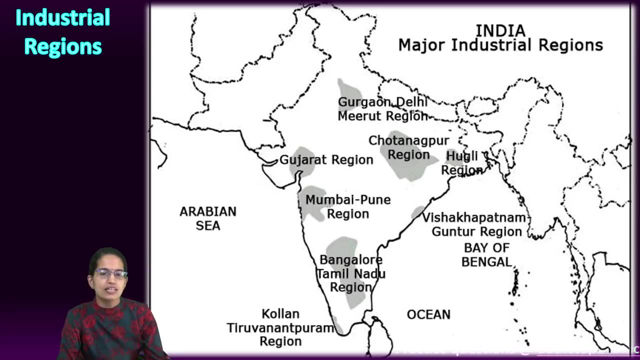 bringing in more investments in India, removing the restrictions and obstacles of trade and encouraging other companies to be established at a much smoother and easier pace. So what are the major industrial regions in India? As you can see in this diagram, we have the industrial regions seen in the north as well as south. 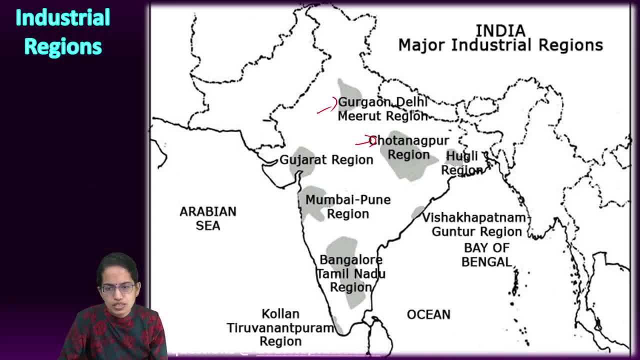 So Gurgaon, Delhi-Meret, Chhota, Nagpur region, Ugli region, Gujarat, Mumbai-Pune, Bangalore, Tiruvananthapuram and Visakhapatnam-Guntur are some of the major areas. 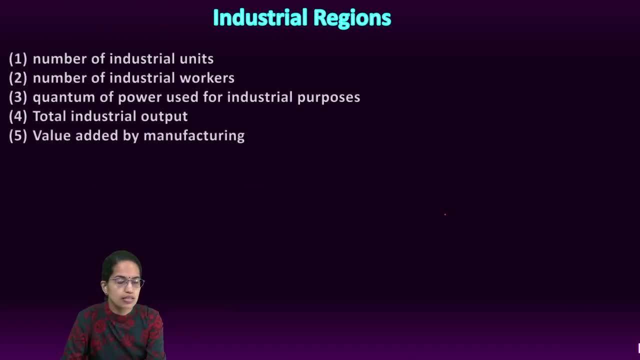 which are the major industrial clusters in India. But let's understand how these industrial clusters are defined. So the first is: how many industrial units are there, How many industrial workers are there? How much power is utilized for the purpose of industry? What is the total industrial output from the region? 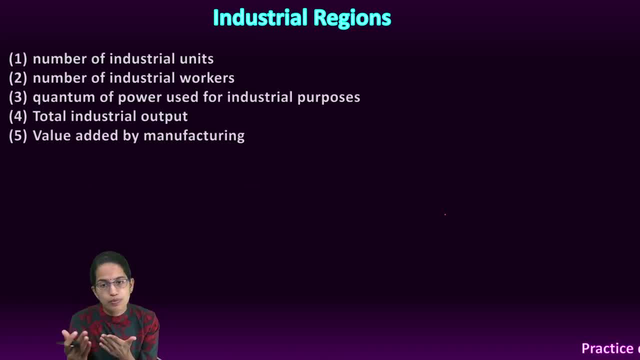 And is there any value addition to the process of manufacturing or by the process of manufacturing which brings in a substantial difference, would determine whether that cluster would be called as the industrial cluster or not, or the industrial region or not. So based on these five parameters, we identify the different areas. 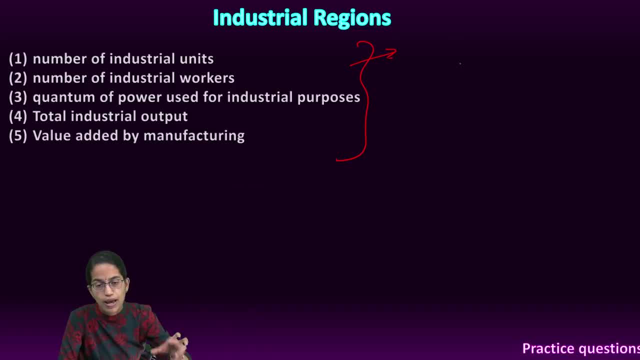 And what would be the areas we have already understood in that map. So the first one is the Mumbai-Pune region. Now, Mumbai-Pune was originally meant for cotton textile. Again, Mumbai was a port area and with the opening of Swiss canal in 1869,. 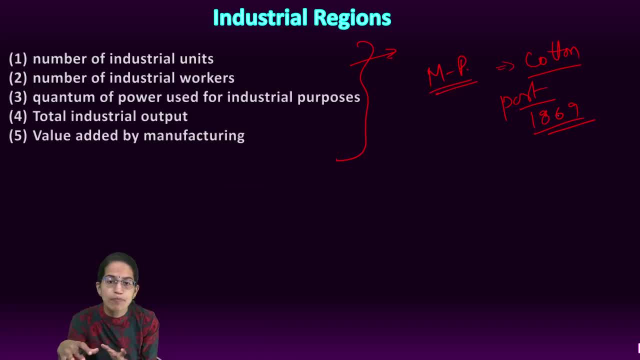 it brought a significant impact onto the port of Mumbai, with more trade and more opportunities. A lot of material was imported and exported through this port, So definitely development of the Mumbai-Pune cluster started Now again. this region had significant amount of hydroelectric power project. 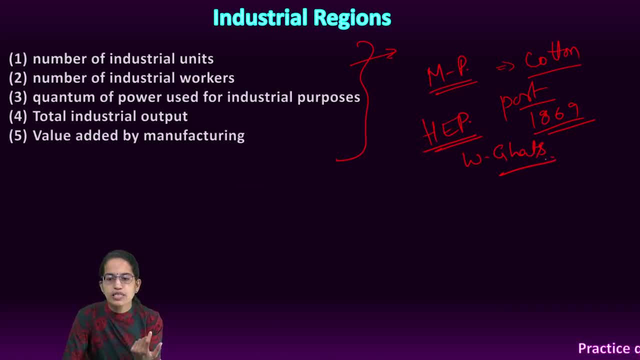 which was the result of Western Ghats. With the Western Ghats, numerous rivers and tributaries draining, you had numerous hydroelectric power projects which affected the area. Besides cotton textile, this region also is known for chemical industries, petrochemical industries, leather industries, synthetic industries. 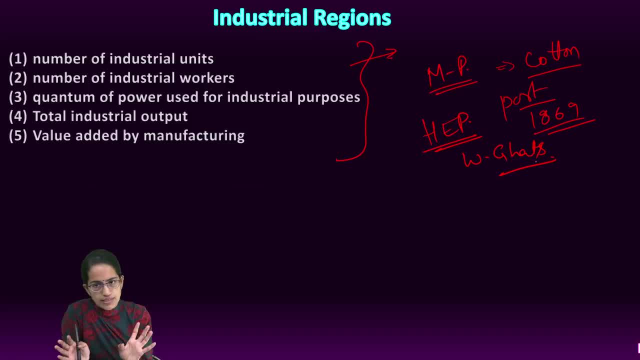 plastic goods industries, electrical shipbuilding, as some of the major industries. The next important is the Hooghly area. Now, Hooghly area lies from Bansbariya in the north to Birla Nagar in the south, And then again you have Medinipur in the west. 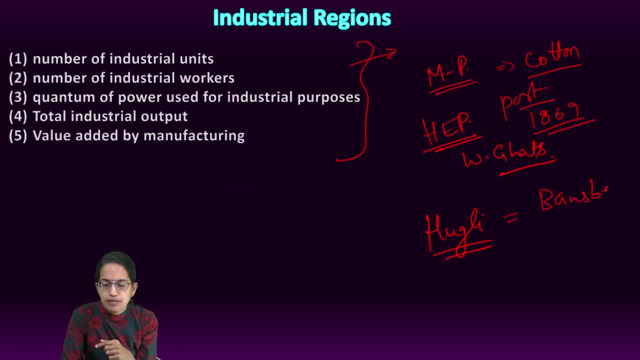 So that is the extension. So it's Bansbariya in the north, Birla Nagar in the south, and then in the west it is Medinipur. So these are the areas where you have the Hooghly cluster. 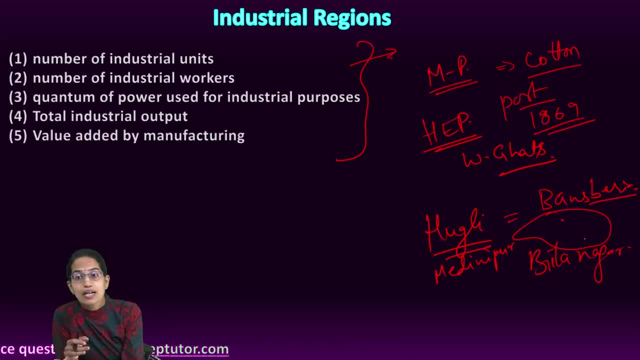 Now why Hooghly cluster was important: Tea plantations from Assam, indigo cultivations from region of Bihar, jute mills from the Rishura region, all these were transported and were the major areas through which Hooghly industrial region developed. 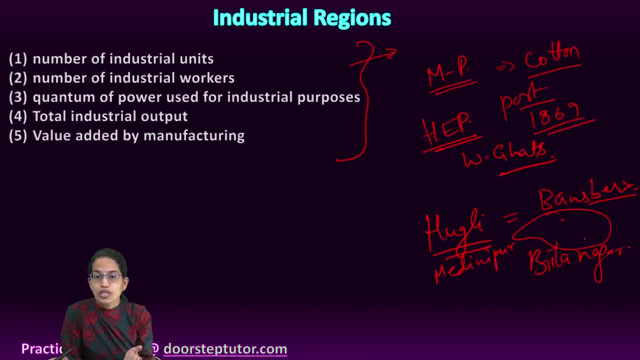 Also, this region had an ample opportunity of change. There was an ample opportunity of cheap labour coming from the regions of Bihar, Odisha, eastern Uttar Pradesh. Now, besides this, what kind of factories were established? Factories were established. The most important here was Hindustan Motors Limited, established at Kona Nagar. 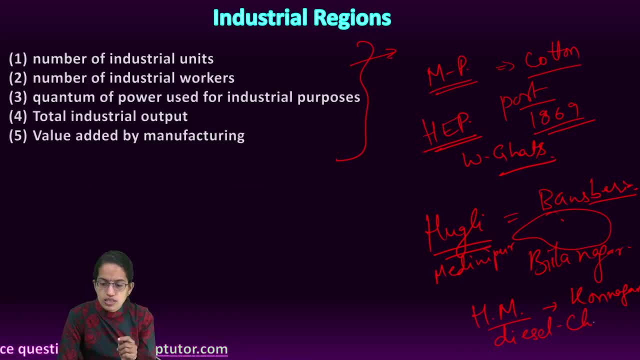 Then we had a diesel locomotive at Chitranjan, So Chitranjan diesel locomotive was another important plant. Petroleum refinery at Haldiya was established And then the nearby centres of Kolkata, Haldiya, Serampur, Rishra, Bansbariya, Hooghly Belar. 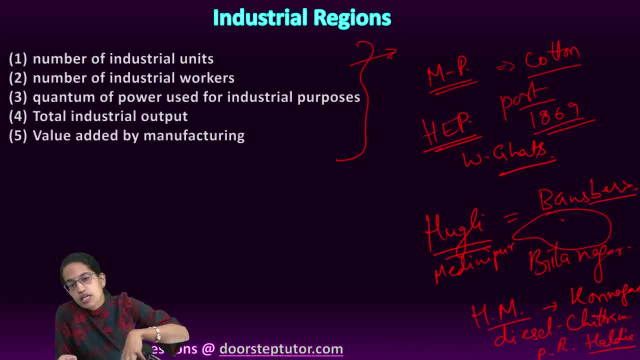 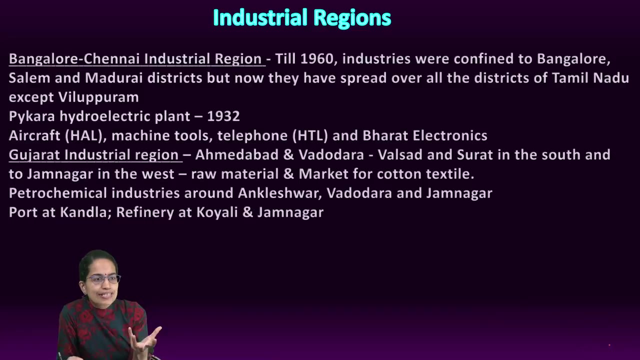 Belur were some of the areas which developed because of the Hooghly industrial region. So Mumbai- Pune industrial region started with cotton. Hooghly initially started with tea, indigo jute mills and later expanded to other plants. The next is the Bangalore- Chennai industrial region. 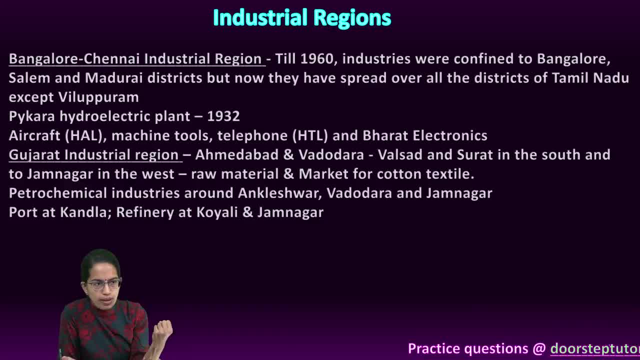 So till 1960s industries were mainly confined to the Bangalore area, Selam area and Madurai area, But slowly this whole belt started to develop. The most important hydroelectric power plant here was the Pekara hydroelectric power plant, which was established in 1932.. 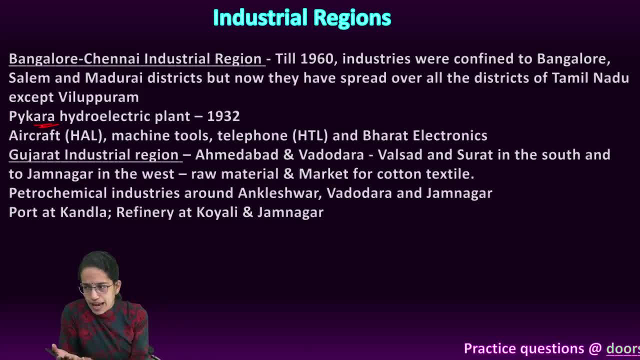 What kind of industries came in? Textile wagon, matchbox, leather goods, light industries, medical industries, aluminium, sugar, cement, glass, fertilizers, paper were some of the industries. Some of the major centres which developed were Hindustan Aeronauticals Limited, HAL plant. 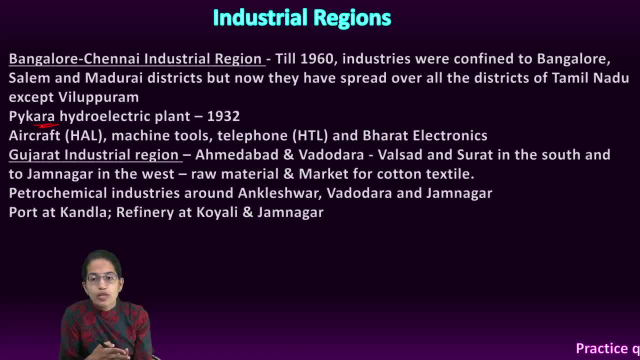 HMT, Hindustan Machine Tools, Telephone Line, Hindustan Telephone Lines, Bharat Electronics were established. So Bangalore, Chennai industrial area developed. The next was the Gujarat industrial area, Here from Ahmedabad and Vadoda, Valsad and Surat in the south, Jamnagar in the west. 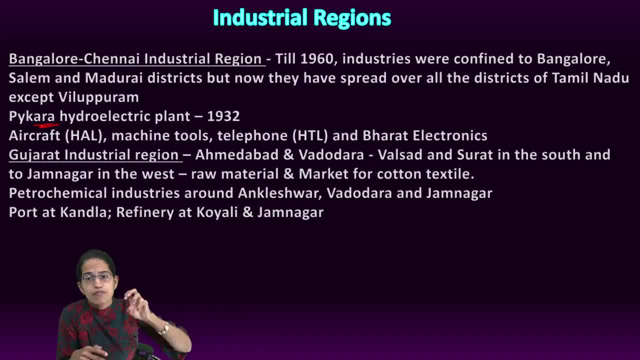 whole of this region was a centre for raw material as well as market for cotton, Not just cotton. textile Petroleum refining started at Jamnagar, Koyali. Then we had petrochemical industries at Ankaleshwar, Vadoda, Jamnagar, which were established. 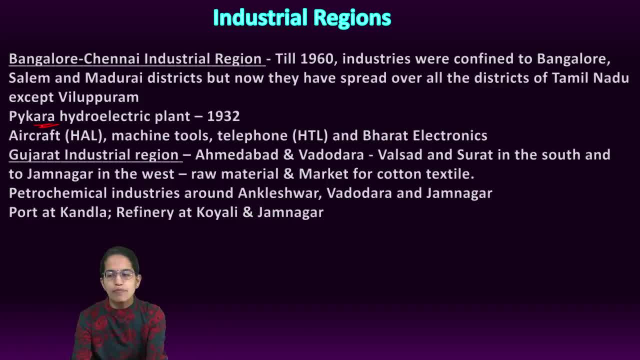 Besides these cotton, textile industries, petrochemical industries, dairy products, food processing, pharmaceuticals, dyes were some other industries which came up. So the whole area of Ahmedabad, Vadoda, Surat, Rajkot, Surendranagar. 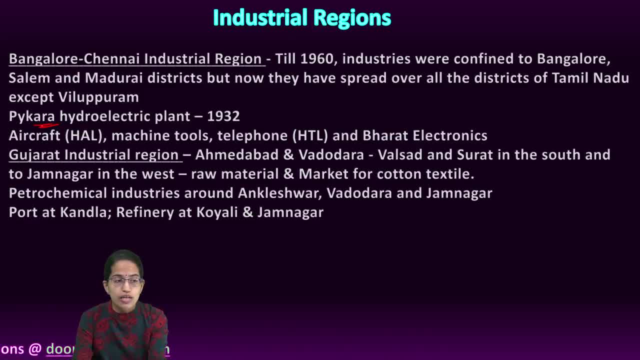 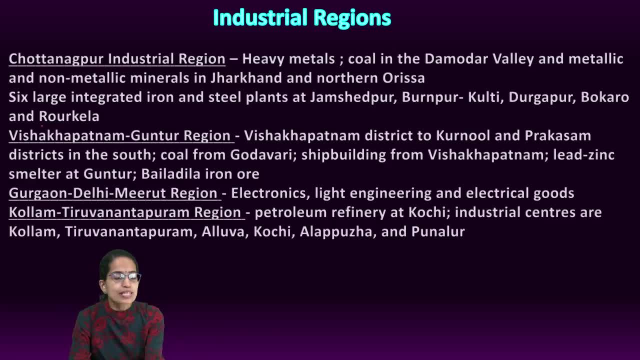 Khera, Jamnagar were the areas where Gujarat industrial regions started to prosper And with the proximity to port this was further eased. The next important sectors are Delhi, Meerut and Gurgaon. Here electronics, light engineering and electrical goods industries were established. 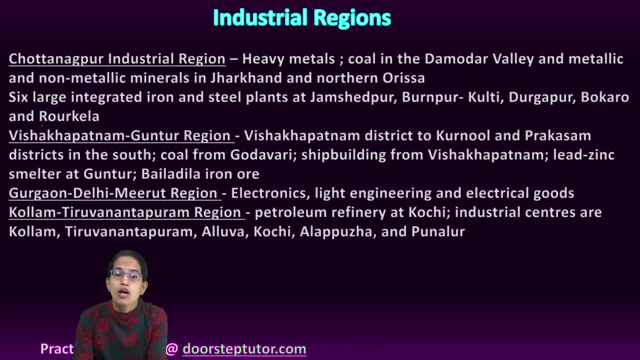 Usually what we call as the footloose industries. Also in the nearby areas of Punjab we had the woolen industries, So cotton, woolen, synthetic, hosiery fabric industries In the south Kolam, Thiruvananthapuram region. petroleum refinery was established at Kochi. 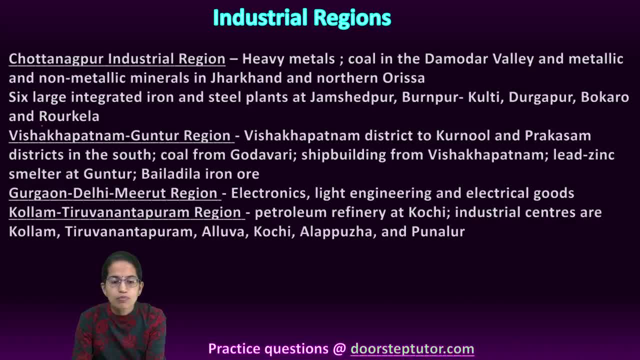 Industrial sectors at Kolam, Thiruvananthapuram, Kochi, Alapuzha and Punnalur were established. Major industries were mainly the sugar industry, rubber industry, then we had the coffee industry, fertilizers, fish based industries, aluminium industry, cement industry as the major industries which were established. 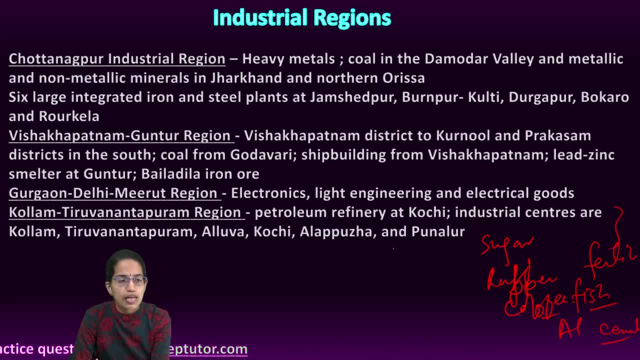 In the Kolam Thiruvananthapuram region in Kerala In the Vishakhapatnam Guntur area. Vishakhapatnam district to Kurnool Prakasham in the south were the major centres. So shipbuilding in Vishakhapatnam we had the Vizag steel that was established. 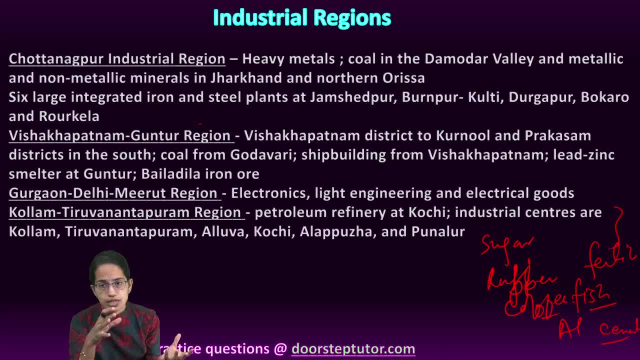 Coal was brought from Godavari Lead and zinc smelter plants in Guntur area, Bella della iron steel plant, from where iron was obtained. So this whole area of Vishakhapatnam, Guntur, Kurnool, Prakasham.